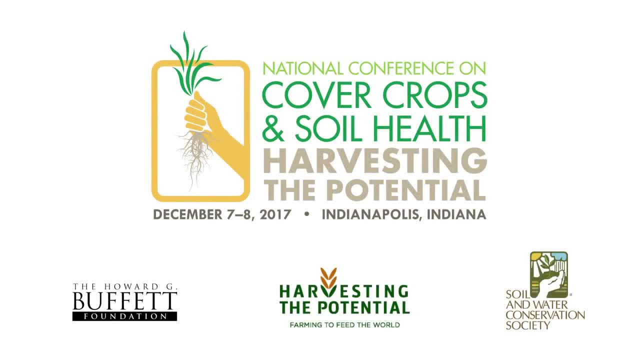 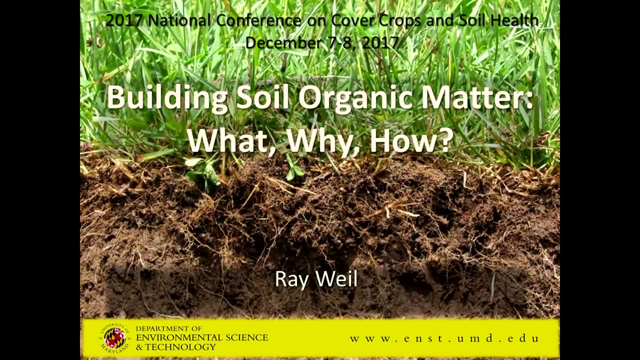 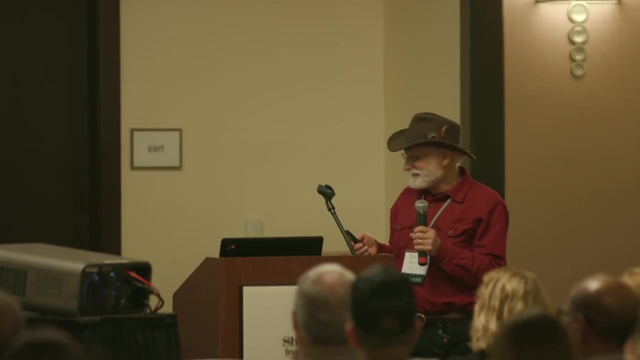 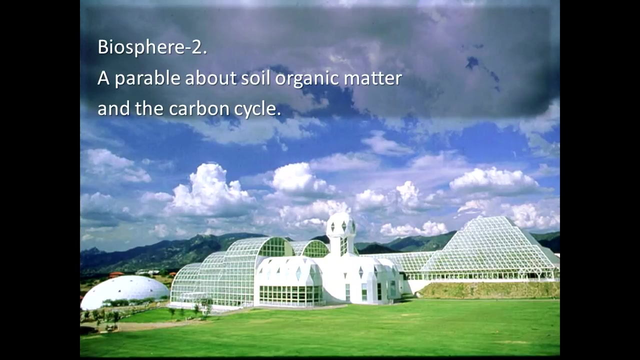 So I'm going to start out breaking whatever rules I can, right? After all, this is a revolution, right? I really didn't know where to start with this. I was teaching until about 5.30 yesterday evening in College Park, Maryland. 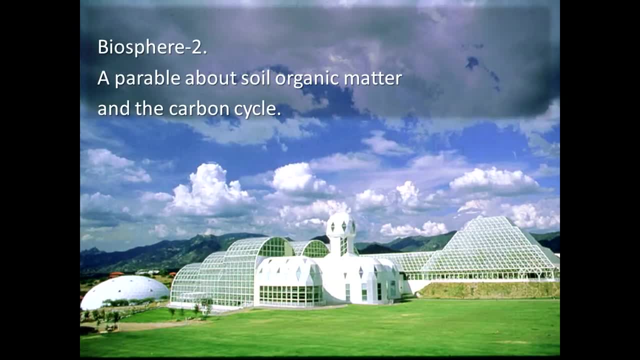 It was the last day of the semester so I couldn't very well leave, And by the time I got into the hotel and hit the bed it was about 2 in the morning, So I'm not totally here. You know what Uber wanted to charge to get from the airport to here. You know how Uber takes advantage of you, right? $175 is what the Uber price was. I found a taxi for $75, so we're doing all right. I want to start with this. Some of you may have visited this place. 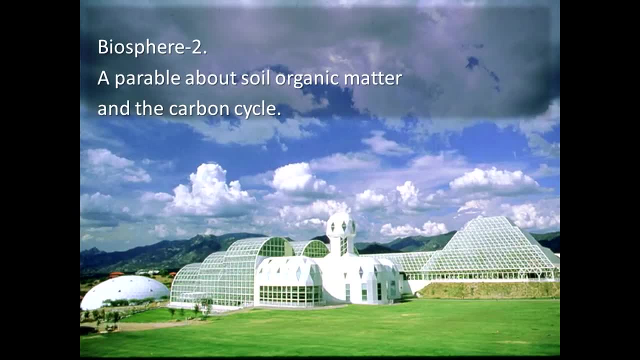 It's become kind of a tourist attraction. It's in Arizona, out in the desert. although, first off, what are they doing with all that grass growing in the desert? right, Well, that's because they're obviously not too smart ecologically. 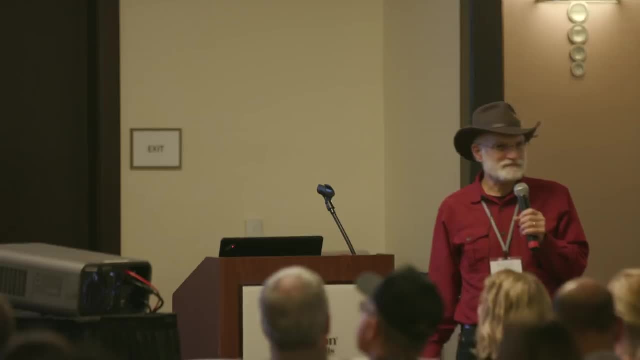 But this was supposed to be the pinnacle of our ecological knowledge. This was started, oh gosh, about 30 years ago. A wealthy individual invested in this first. It then got taken over by a number of universities and research groups. It's called Biosphere 2.. I never really found out about Biosphere 1, but it's basically a gigantic sealed greenhouse. It includes some lungs that expand so that when the air pressure changes the greenhouse volume can change, so they can keep it sealed And they think. well, right, we know so much about ecology and how the earth works. we'll be able to really learn if we sort of make this mesocosm. 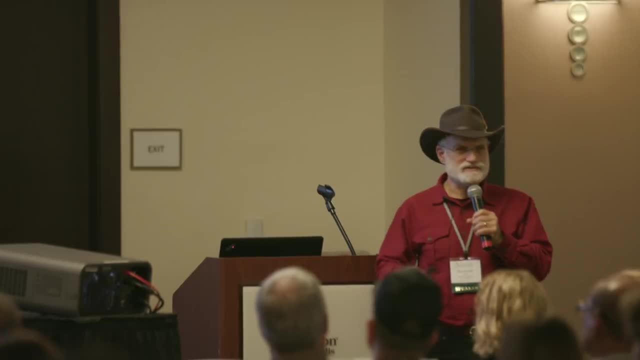 We can create this world And we're going to monitor everything and monitor all the gases and seal it up And we should be able to create a balanced system. You know, plants produce oxygen and animals use it And they had different biomes. 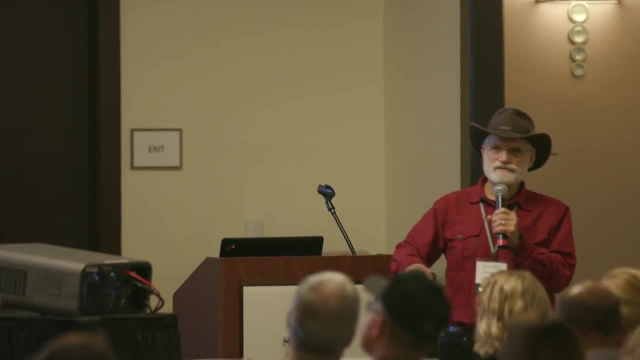 And some of these greenhouses were oceans and some were tropical rainforests and some were grasslands and some were agricultural And it was very complex And then they put some people in it. They called them biospherians. They had a team of young scientists. 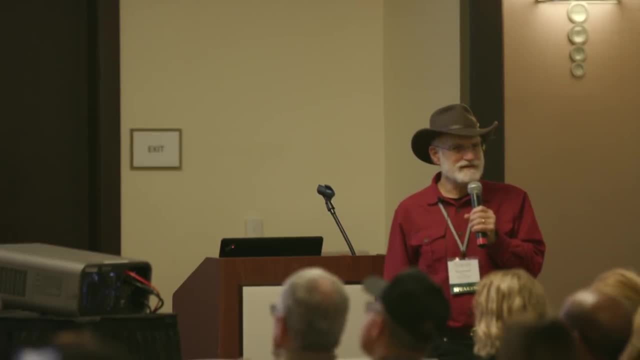 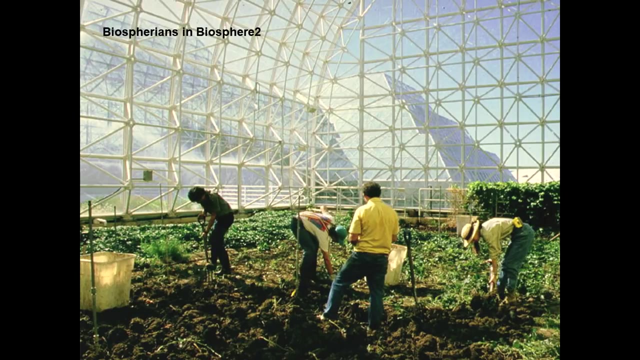 And this is supposed to be all sealed up. After all, it's a balanced. It's a balanced ecosystem, So part of their job was to grow their own food. They weren't sending anything in. All right, The water gets recycled. 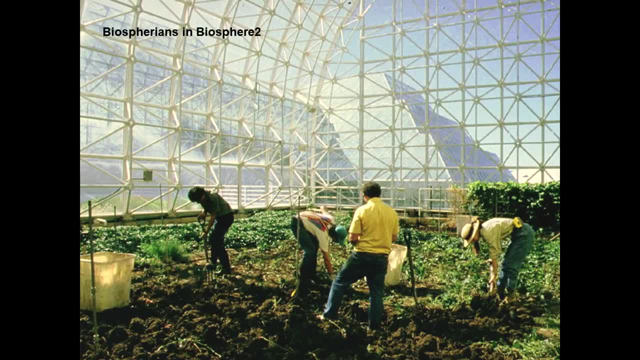 The air is recycled. Well, first thing, these people found it was really hard to grow your own food. Has anybody ever tried that? I had a grad student who many of you know, Joel Groover. Anybody know Joel Groover. 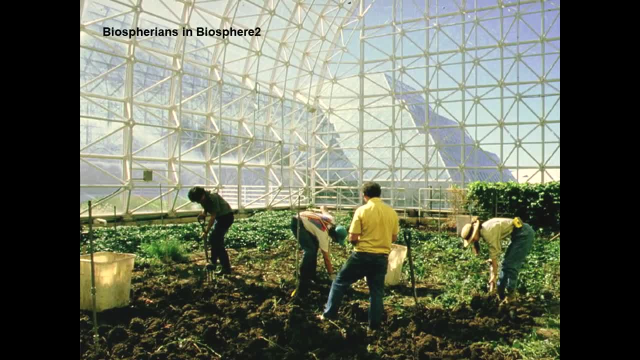 He's not too far from here, Everybody, I'll tell you. I told Joel that lots of hands went up. Well, what an interesting guy, huh. He was my grad student years ago, And one year he came in the middle of his program. 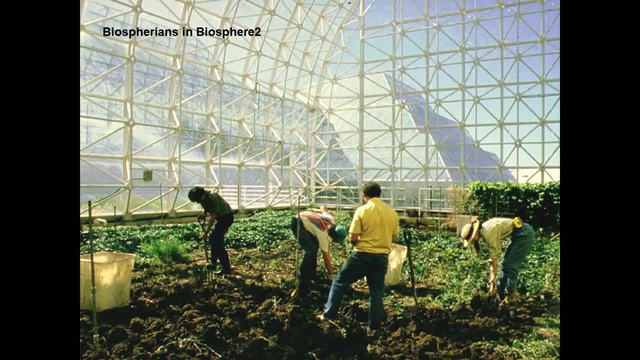 He said: for the next six months I'm only going to eat what I can grow in my garden, That's it. And he had boxes of sweet potatoes and roots and stuff stored in the cooler where we keep our samples And it was an interesting experience. 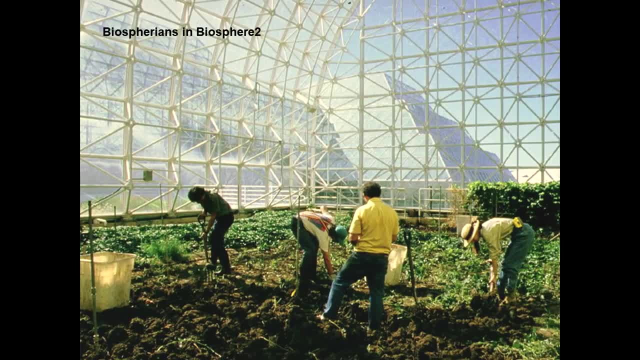 He started losing weight And he stuck with it. So these folks found it was hard. But worse than that, they were in there for a few weeks and they started getting dizzy and feeling woozy And they were sort of getting a high altitude sickness, like as if you were, you know, 15,000 feet in the top of the Andes Mountains or something. 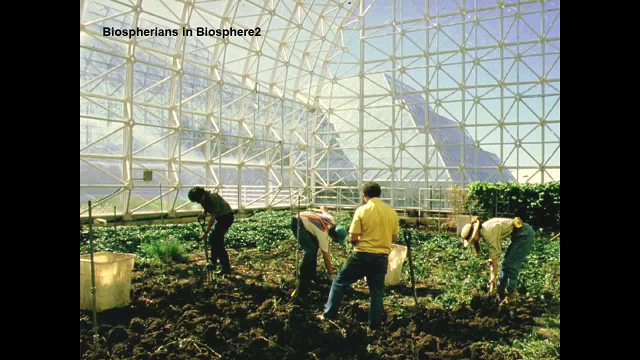 And they're monitoring all this stuff and they're running out of oxygen. The oxygen is getting low. I said, well, we had everything in balance. We had enough plants to produce the oxygen. What was going on here? And these guys forgot about the soil. 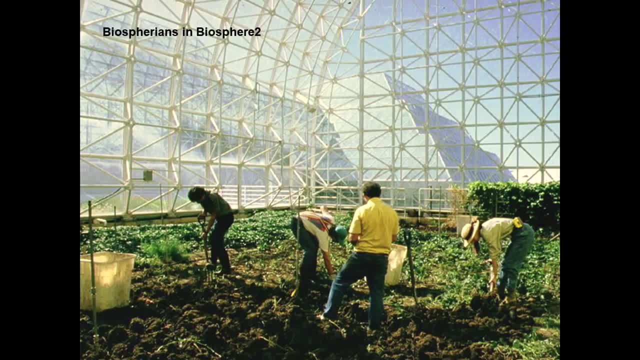 So they wanted to grow plants And so they had to put soil into this thing. So they dug up. there was an old lake bed out in the desert And they dug that up and mixed it with peat, moss and compost, Created kind of a potting mix. 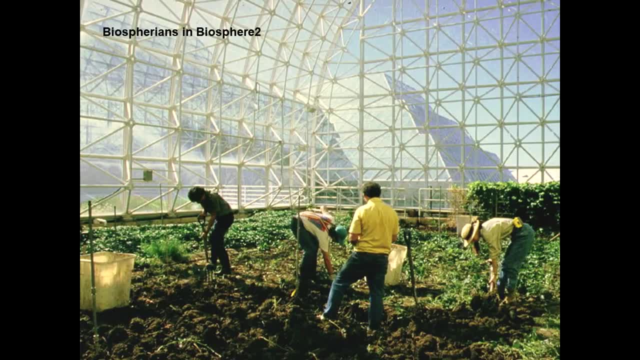 And filled it to about three or four feet deep. Now you know what soils look like. right, The organic matter is at the top. It's not like organic rich all the way down. There's a huge amount of organic matter in the soil. 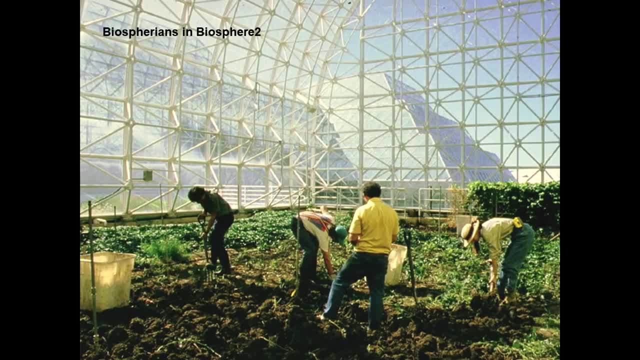 Because that sounded like a good idea And they stuck it in this ecosystem And, of course, all the bugs in the soil went wild And it's the middle of the desert, So it's hot And it's totally out of equilibrium. 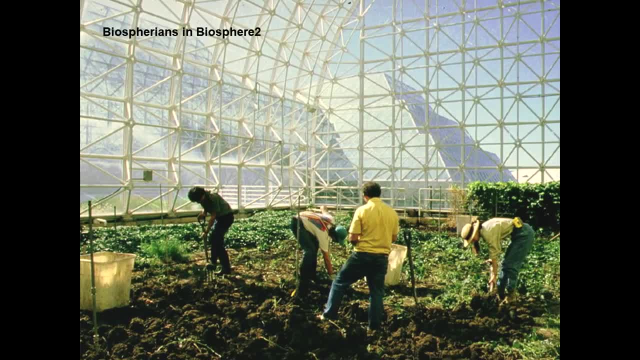 And the soil starts to decompose. right, It's using up all the oxygen, giving all the CO2 up. The concrete, by the way, didn't help either. We often forget about concrete, But you have to carbonate, So they had to cheat. 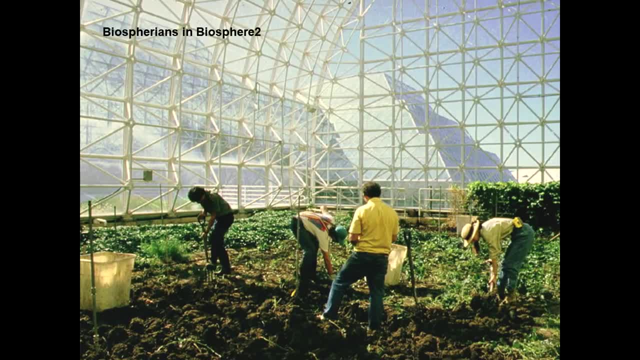 These people were going to die. They had to pump in oxygen and cheat, So this was sort of the best effort. Thought we knew everything. Thought we could create a system. Wasn't that simple? And the big problem was they forgot about the soil. 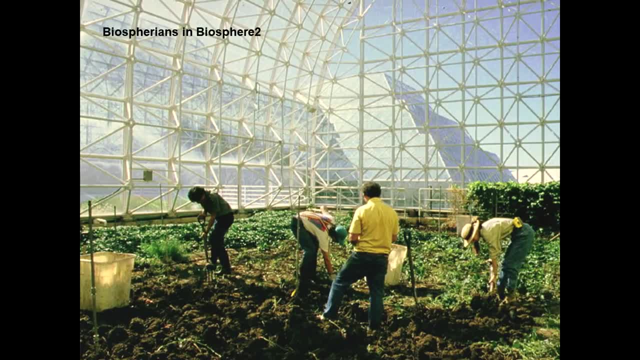 Everybody forgets about the soil. It's just like people that study plants forget about the roots. How much do you know what's above ground and how much do we know what's below ground? Well, it's hard, right. If you've ever tried to study roots, it's hard. 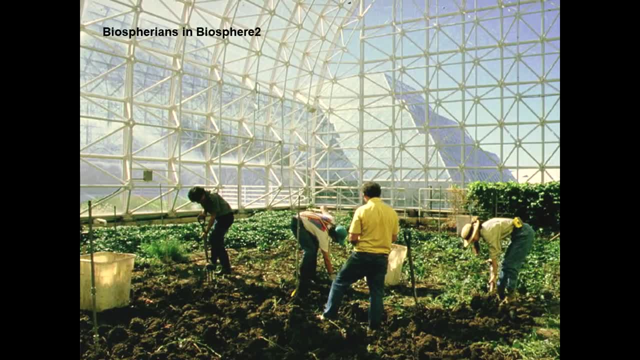 We don't live down there. It's really hard to get samples. Almost nobody does it. They just use some kind of estimate from some old paper someplace And they say: well, we doubled the top, It must have doubled the roots. 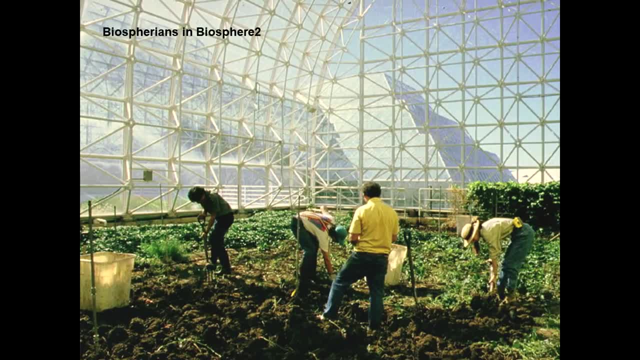 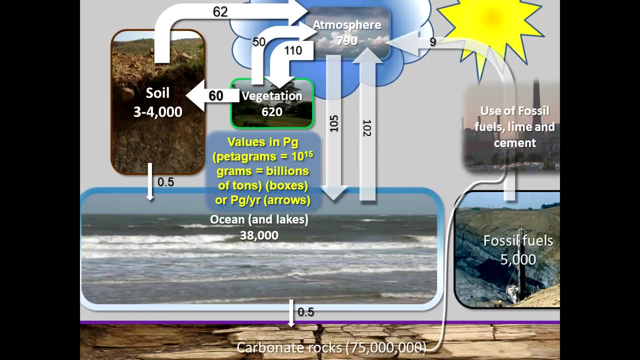 But it doesn't work that way. So soils are a really important part of the whole carbon cycle in the world, Just like that greenhouse model ecosystem. We can't forget about the soil. It's really important If you look at where the carbon is. 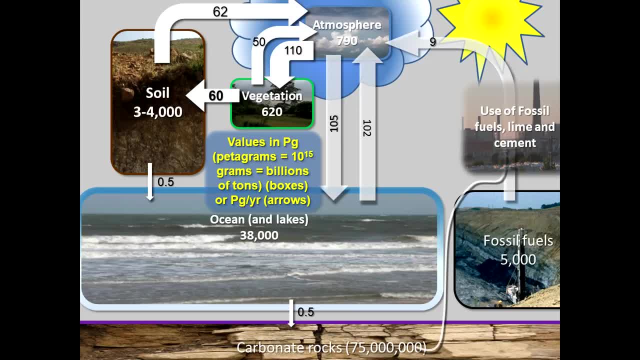 and this is what's driving all this crazy weather and all this increased hurricanes, and the rains come and they don't come, and they come too hard, and all this strange stuff we have going on is being driven by too much carbon in the atmosphere. 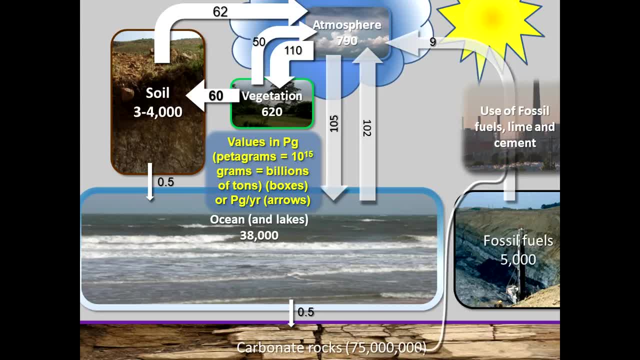 This is the global carbon cycle, And the part of it that's active is up here. It's driven by solar energy, of course, And the vegetation is a part of it, But there's more carbon in the soil, And you hear this statistic a lot. 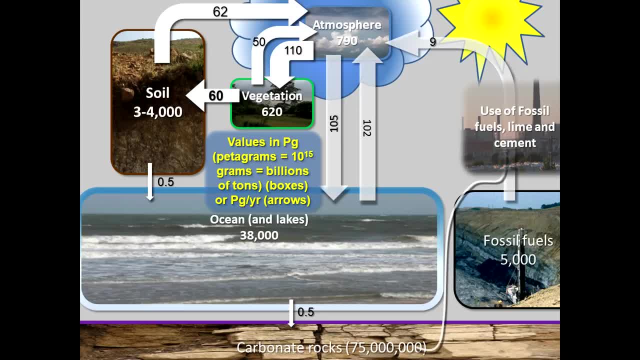 But not everybody appreciates it. The soil is where the carbon is, Depending on how deep you go and what you include. Three or four thousand, These are pedigrams. That's a big number. So there's actually more in the soil than there is in the entire atmosphere of the planet Earth. 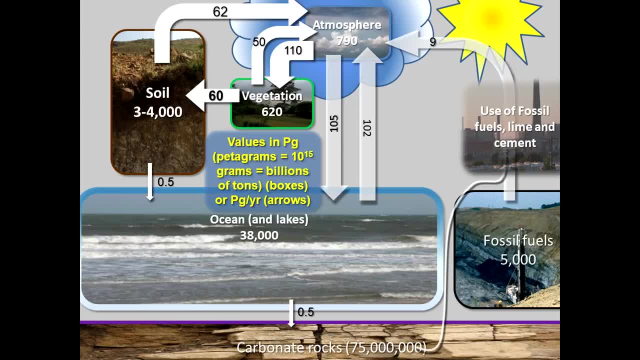 and in all of the vegetation. The soil has been soaking it up and storing it for millennia. So every year there's about 110 pedigrams that are taken out of the atmosphere by the vegetation Photosynthesis And about 50 goes back in by the same plants. 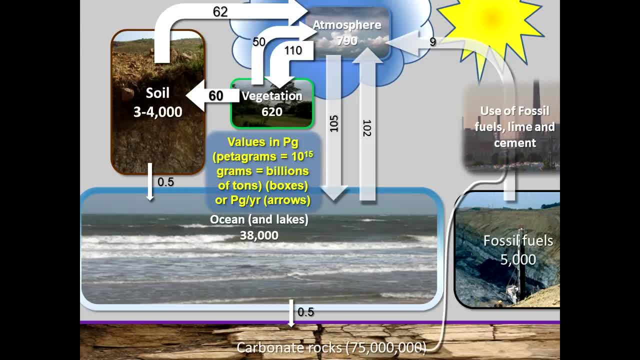 You know, at night they respire Right And most of the difference goes into the soil. That's the dead plants, That's the root exudates. That's all of that. Now, what goes into the soil and what comes out of the soil? 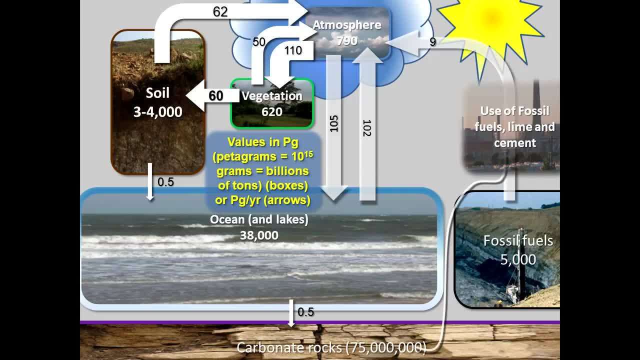 ain't in balance. That's a big part of the problem And that's because of the way we manage soils. It's not just agricultural soils. Part of it's the fact that we've got 7 billion people on this planet and we've cleared more land. 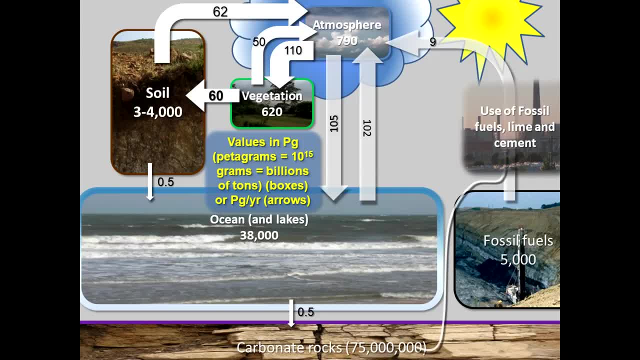 and turned more of it into agriculture, Forests and grasslands than ever before. So every year, the way we're doing it now, the soils are losing carbon. Anybody that's taken cleared natural vegetation in a forest or plowed up the prairie. 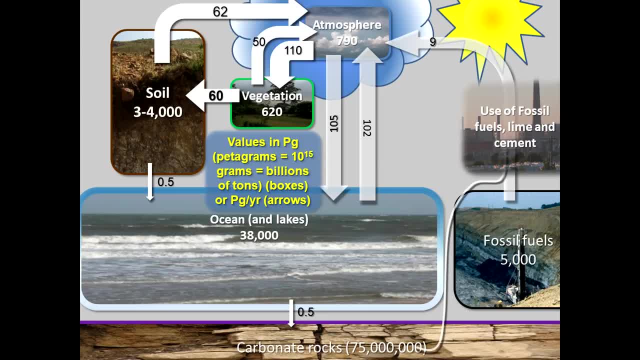 Did I say plow Strike, that That converted, you know, grassland to cropland, Those that under most conditions you start losing organic matter. So what we really need to do is build this organic matter and change that balance. We have to put more into the soil. 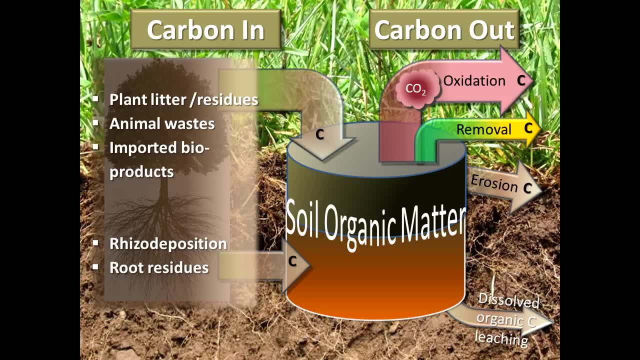 than what the soil is respiring out and is losing. And you saw, it's not that huge a difference, Right? It's not that much in 62 out. It should be doable- I think it is- If everybody were doing stuff. 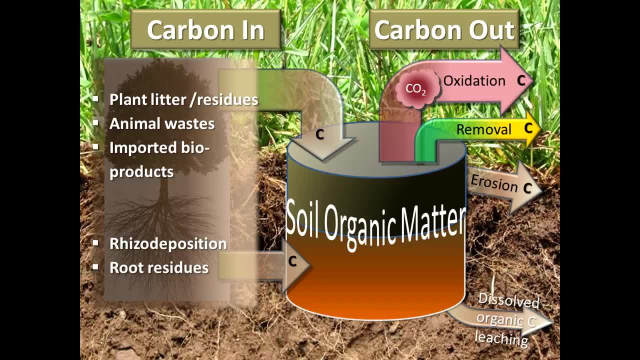 that a lot of the farmers in this room are doing, we'd be making a lot of progress Right. It's sort of scaling up and improving what we do. So organic matter is really kind of an input-output thing. It's like your bank account. 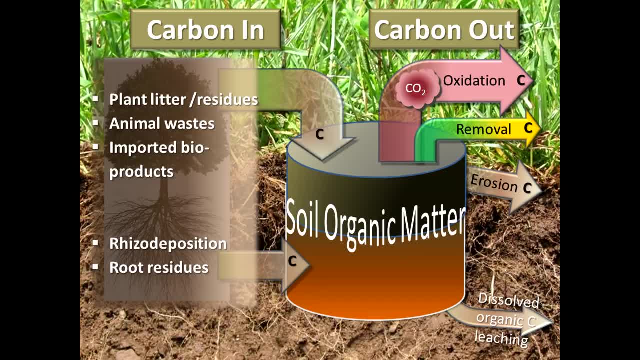 And organic matter has these. you can make a financial analogy. it's a little bit like money. There's a quandary. You can save your money and put it under the mattress, but then what good does it? do you Right? You've got money under the mattress. 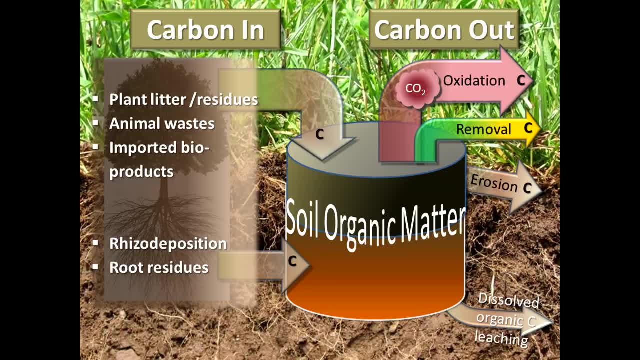 Or you can spend it and party, have a good time, buy a new tractor, a new car, take a trip, and then you'll run out of money. We really want to do both, And we want to do both with our organic matter. 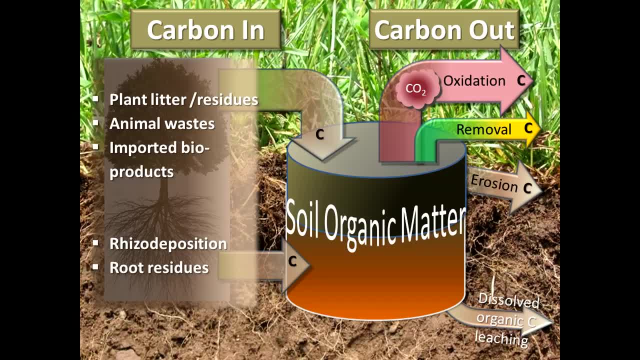 We want to protect it, accumulate it, but we also have to spend it If we want to get the nutrients out of it. if we want to feed the food web, we have to use it. We have to keep it cycling. So let's look at. 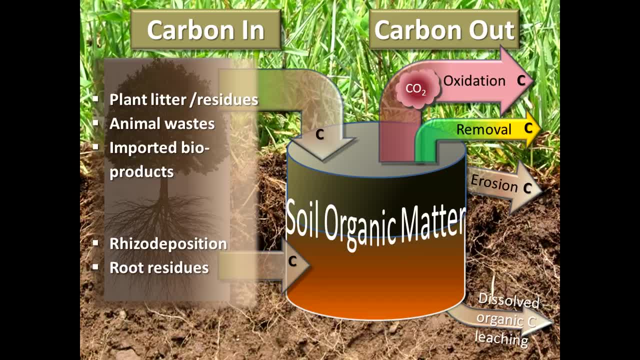 so organic matter is kind of like a tank that we're trying to fill, And most of it comes from plant residues. That's really the only way to fill it. Sometimes we think we can do it by buying organic material- compost- from down the road. 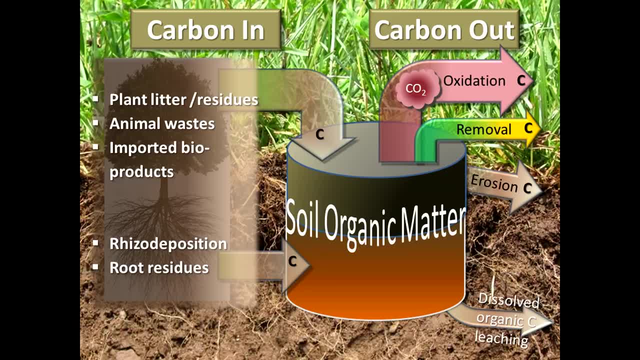 manure from the feed lot or something like that. But in the big picture you only do it by growing plants, And some of that comes above ground, but a lot of it comes from below ground, And the below ground stuff's actually more important. 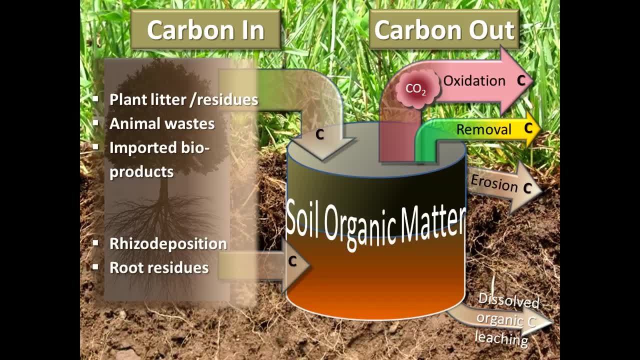 There's a little less of it, but it'll stick around longer and it'll have a bigger impact on soil organic matter, the stuff that comes from the roots. So those are the main inputs: Plant residues, animal waste, manure and riser deposition and roots. 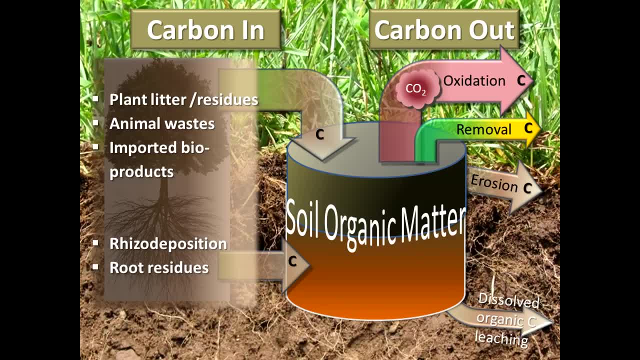 And that has to be balanced with the carbon going out. We need to know what's coming in. We need to know what's going out, so we can make sure that there's always more coming in than going out, as far as we can. Now you get to a point. 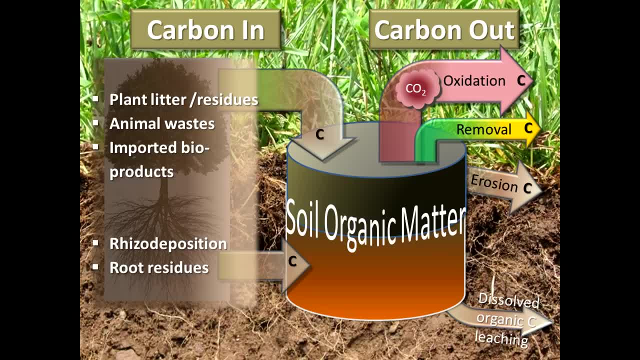 where you're probably going to be in equilibrium, but let's hope that's a really good point right? Most of it's going out by oxidation. All those critters are doing what you're doing right now: digesting your breakfast and breathing out CO2.. 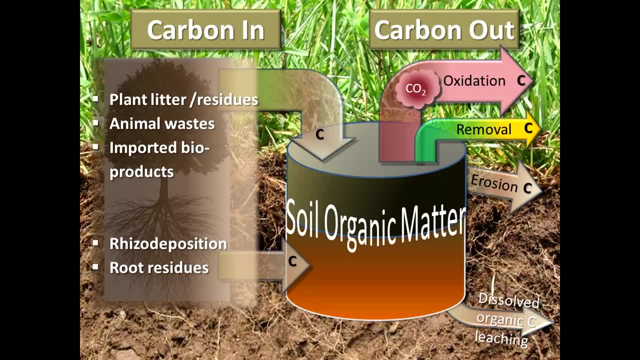 And the soil is breathing out CO2 all the time, which is a good thing. We just have to make sure we feed it enough Right? Some of it's harvested, which is a good thing too, because that puts money in the bank. 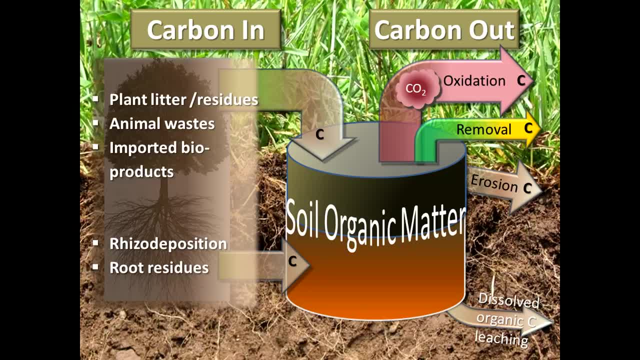 We have to take some of that carbon away. We have to haul out the corn grain or the hay or whatever it is we're taking away. But we have to keep in mind that we're harvesting some of it, But there's no excuse for letting some of it wash down the hill. 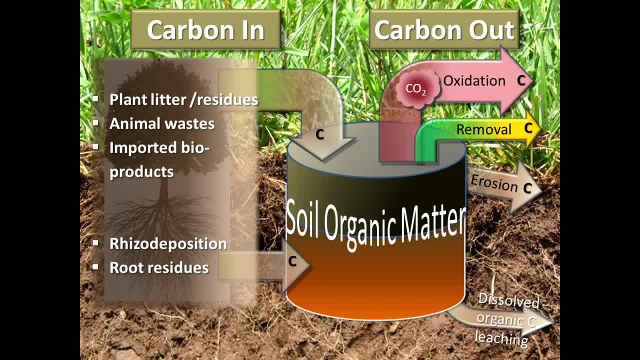 There's really no excuse anymore. 10,000 years of agriculture. we didn't know how to control that, but we know how to do it now right? I think there's folks in this room who probably have seen that difference during their lifetime. 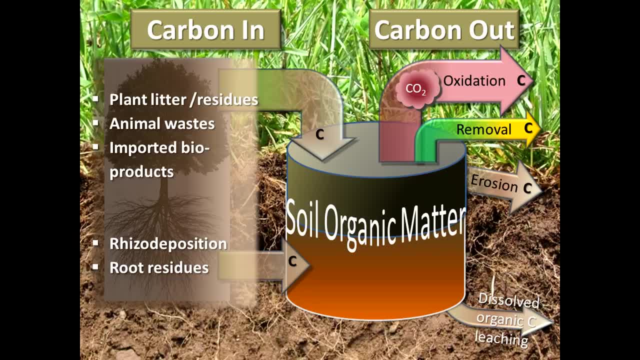 and they don't worry about erosion anymore because they know how to control it. It doesn't happen on their farm- Virtually none, When you're doing no-till and cover crops and minimal disturbance, keeping that residue mat on the surface. erosion is ancient history. 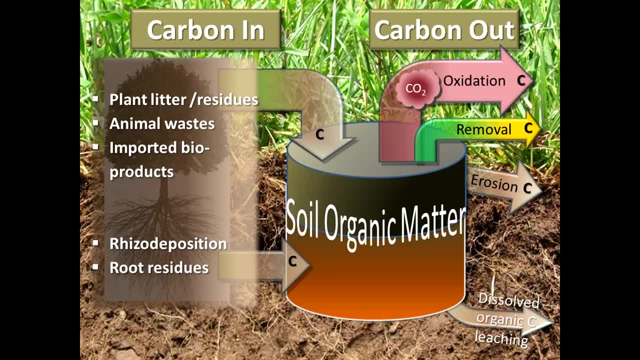 You're almost as good as a forest, But not everybody's doing that. So I hope NRCS, for instance, doesn't forget their erosion message in their drive for soil health. Erosion is still important in lots of places, Maybe not so much in this room. 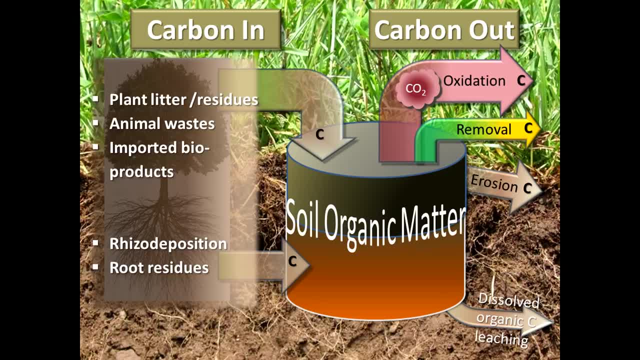 Some of it leaches out with the water. It's dissolved organic carbon. It goes down into the groundwater and there's a certain amount of that. That's a natural process. In fact, that's one of the main ways forests, the natural systems, lose their carbon. 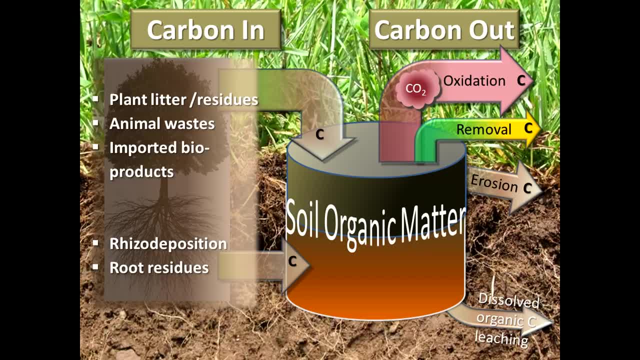 So we have some control over the ins and the outs, Just real quickly. Again, it's kind of an input-output. It's like a tank: You've got water going in and you have a drain And we can control the level of that organic matter. 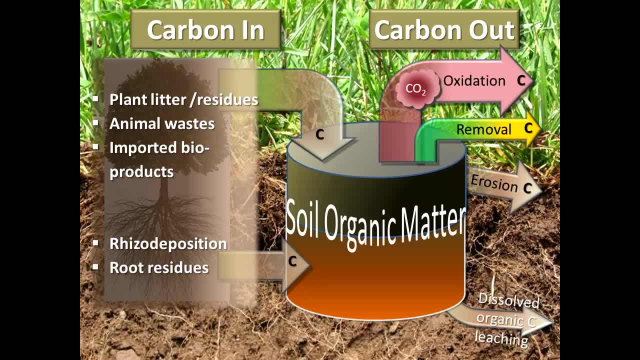 the level of that water by whether or not we have the drain wide open And what opens and closes the drain. the biggest control on that is how much we physically disturb the soil. That's where no-till comes in, So we want to conserve the soil. 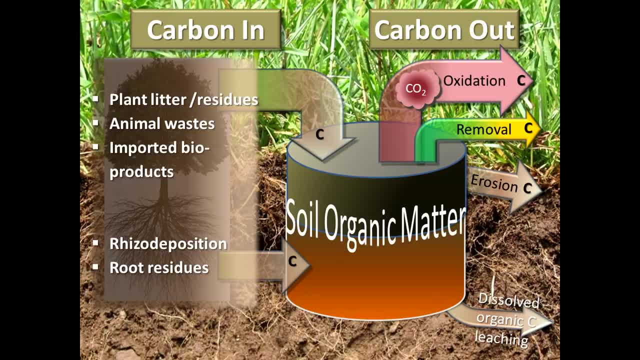 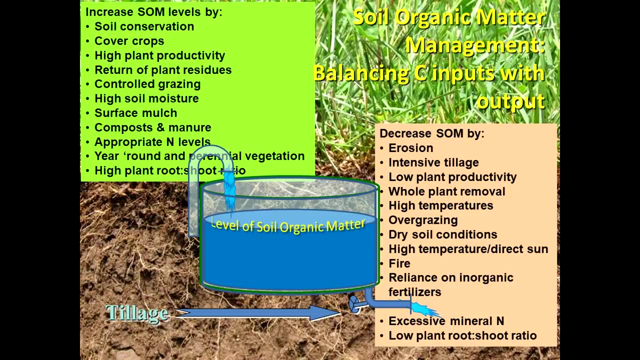 We want to grow cover crops. Cover crops is just adding more photosynthesis, taking more carbon out. that wasn't being done before, right, So it's an added input. And we want to have high productivity If we have low fertility and poor management. 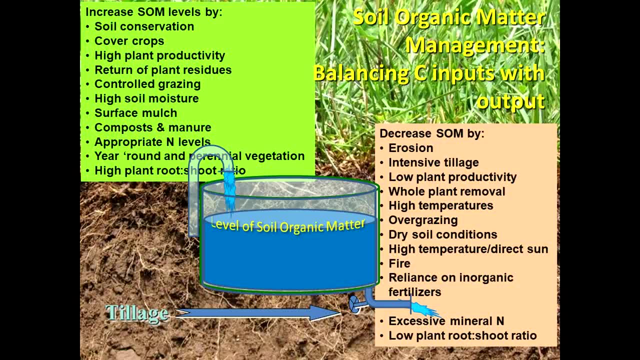 low input agriculture is not conserving anything. There's plenty of low input agriculture all around the world. I work all over the world with poor farmers that can't afford inputs. They can't afford inputs. They're working under marginal conditions And their soils are going downhill fast. 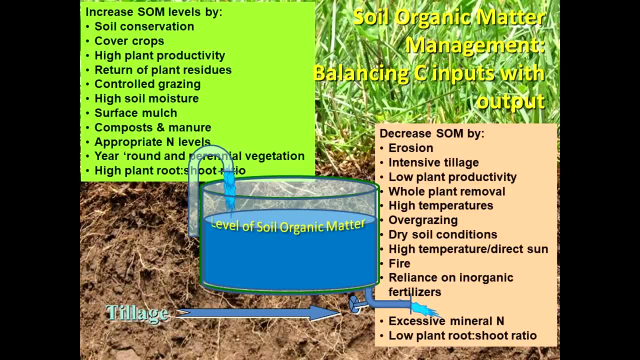 literally and figuratively. You of course need to return the residues. That's a question If you're doing biofuels. you have to keep this in mind. There's lots of work that shows if you take all the residues off. 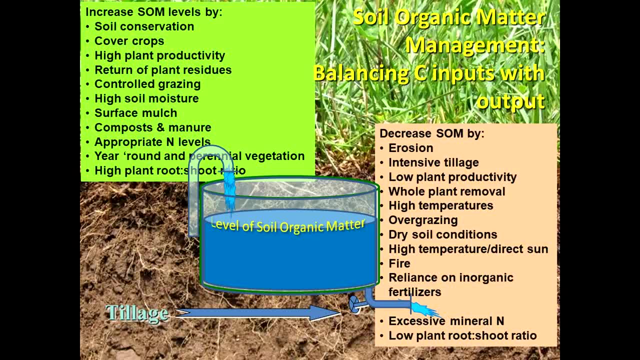 or something like silage very hard on the soil and it happens quick. You start taking that residue off, you start bailing it and selling it and it does not take long- I mean it just takes a year or two- before you start seeing things like infiltration decreasing. 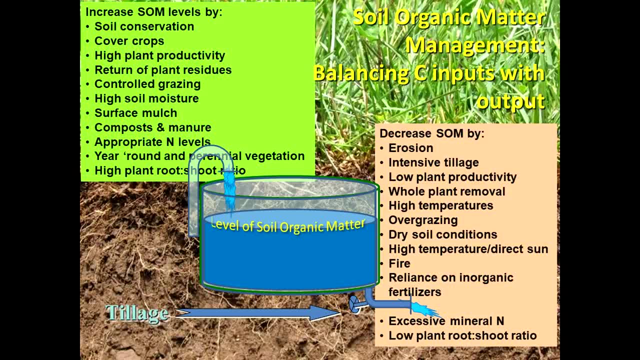 and your soil fertility going down, and pretty soon your crop production is going to go down as well. So you really have to balance the value that you get from those residues and how much you can afford to take off. You pretty much need to leave at least a third of the production. 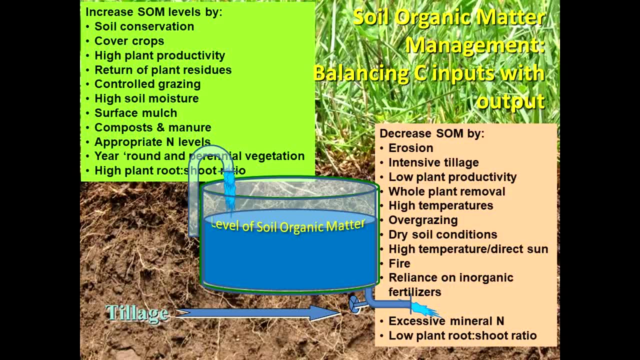 above-ground production on the soil. Managing is great. You know cows get a bad rap. Cows are not a really bright animal- those of you who work with cows, They're not the brightest If you let the cows do the managing. 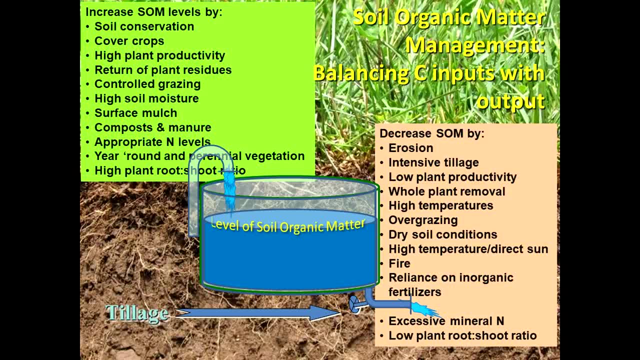 which is what most ranchers and farmers do. they don't do a very good job of it, But if the farmer does the managing in a really intelligent way, controlled grazing is a benefit to the soil and a benefit to the ecosystem and a big benefit to the farmer's bottom line. 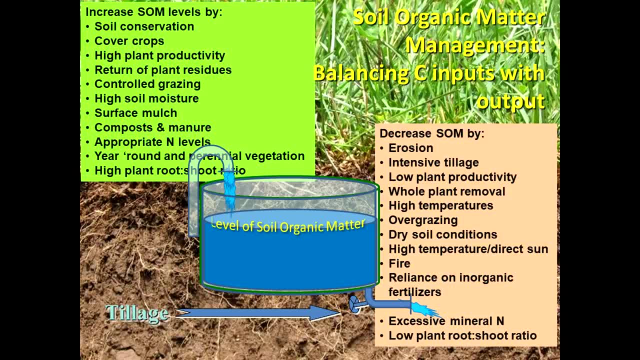 We could do a whole session on that. if you want to talk about building soils, You want to maintain moisture in soils. organically, It's very closely related to moisture. All those processes need moisture. Keep that surface mulched. I've already had a lot of things. 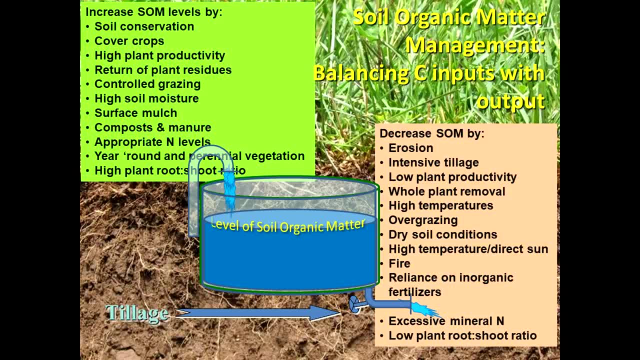 Appropriate N levels. I'll talk about that a little bit more in terms of Jennifer's Goldilocks story and the sweet spot. That's exactly right. Year-round vegetation And people often say, well, we only had six months of vegetation. 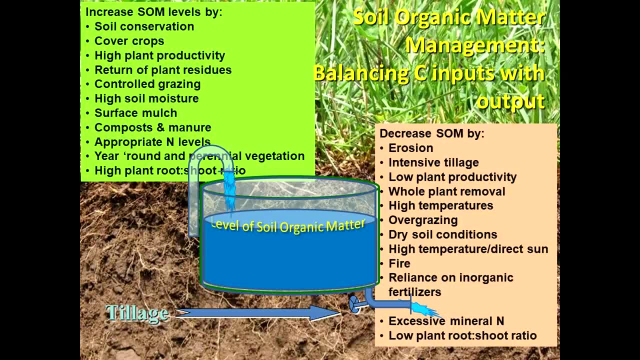 in a corn-soybean rotation. Is that true? Six months? What six months? Tell me what six months. you've got active roots and covered soil with green vegetation in a corn-soybean rotation. Which months Is your field covered green? 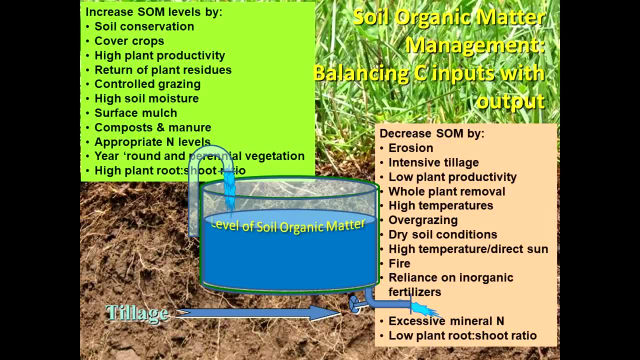 Can you see the land in April, In May? When is it completely covered? When do you have roots all over in the soil? When do you have vegetation? When do you have updated soil? Probably June, right In July. it looks great. 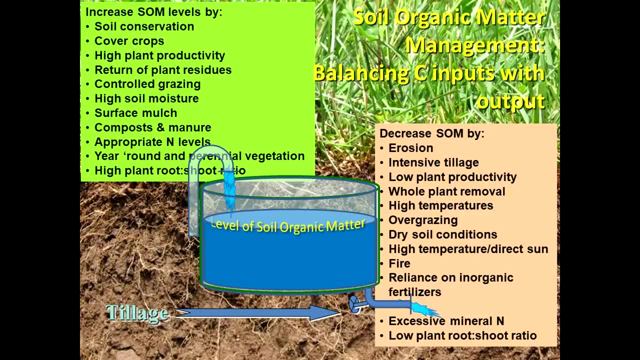 August pretty good, But what about the end of August? Does it start to senesce, Start to mature? What do you think is happening underground when you see those leaves yellowing in the bottom of the plant? The roots are dying. 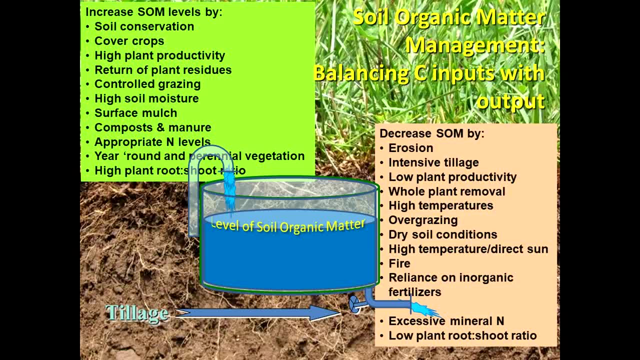 The nutrients. basically by the end of August, nutrient uptake is all done, Maybe into September- It depends on your growing season- But a long time before you harvest. So really it's June, July and August, It's not six. 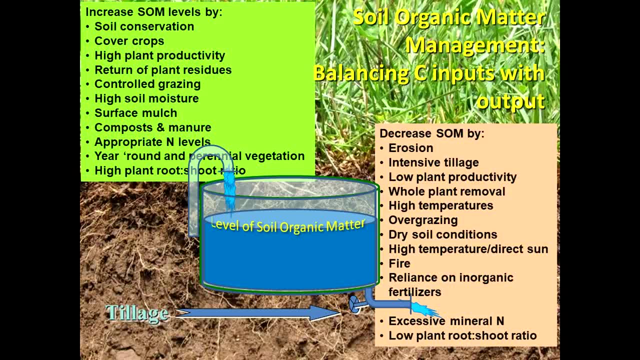 It's three months By September. you've just got dead and dying plants out there. The roots are no longer doing much And they're just sitting there. So you've got three out of 12 months in the typical corn-soybean rotation. 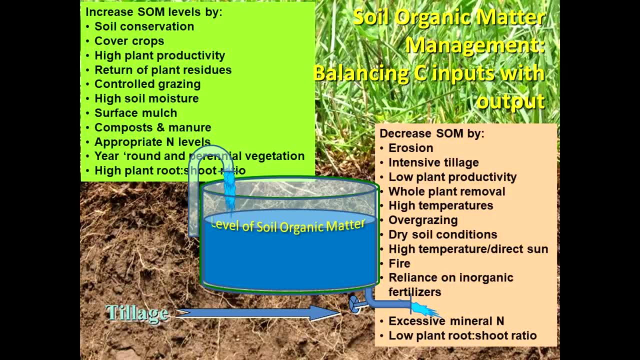 And we need to get those cover crops in. while the crop is still there, While that dead crop is sitting there drying and getting ready for harvest, we want the cover crops coming up and the roots repopulating Stuff. not to do, of course. 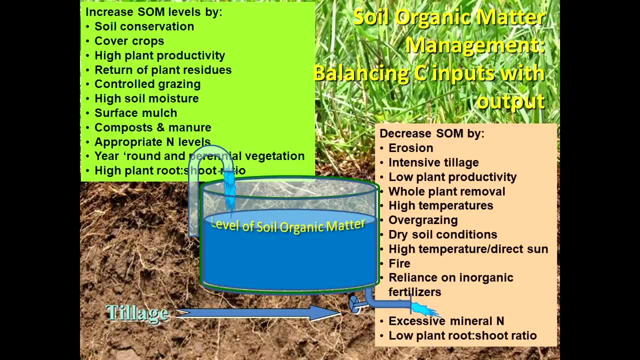 erosion is the worst number one. Don't forget about it. It's not a dead issue on most farms: Tillage, But also low productivity, Lots of problems, Fire. There's still lots of places where they burn crop residues. Did you do that in Kansas at all? 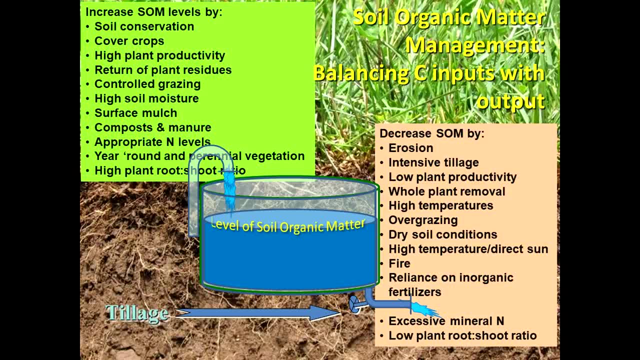 Yeah, Okay, What can you say? Total reliance on inorganic fertilizers. I'm not saying inorganic fertilizers aren't a good thing, But when you're totally relying on it, to the point where you're excluding any organic sources. 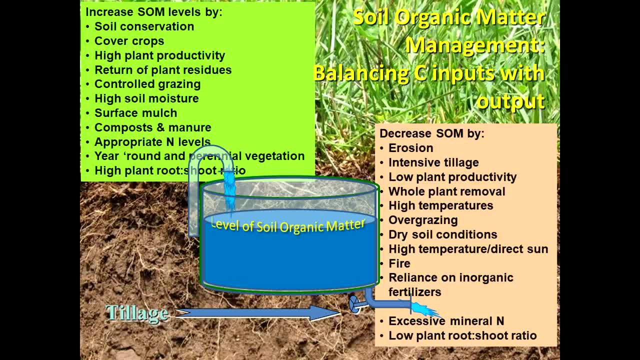 then it could be a problem, Especially with excessive mineral nitrogen And using plants that don't have a lot of roots, Which is sometimes what is actually aimed for. I've seen engineer types figuring out this biofuel business and say: well, we want plants where we can harvest. 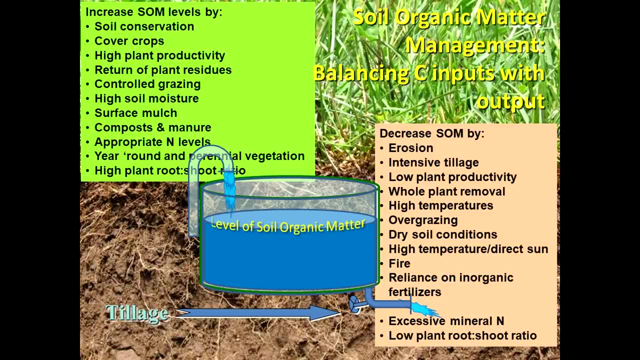 We don't want them wasting. We don't want them wasting all that photosynthesis energy and putting it into roots. We want to have sort of the minimal roots that'll support a plant And then so we can harvest everything and send it to the ethanol plant right. 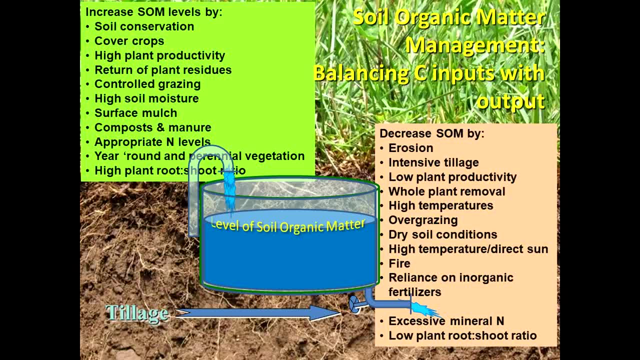 No, I don't think you're going to get too far with that strategy, But that's what they're working on. And then we have sort of the hard fact that most of the carbon that we put into the soil, whether we're putting it in with a cover crop. 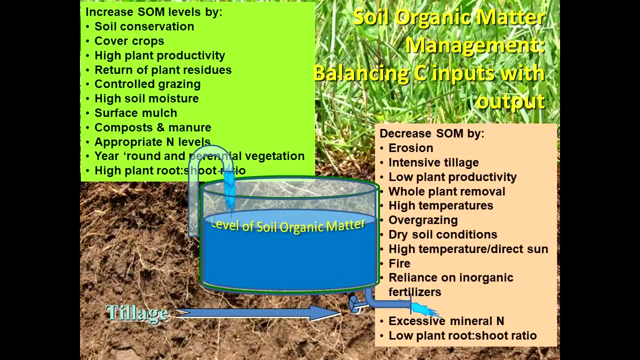 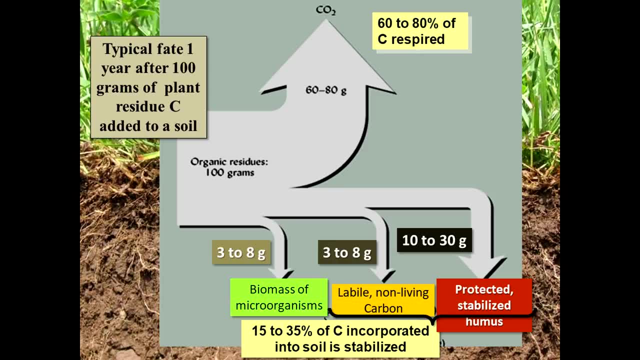 or with compost or whatever. mostly is going to get respired, It's going to get eaten. It's food for all those creatures we were talking about. Some are more efficient than others, So some of them breathe out more of it. Some of them grow on more of it. 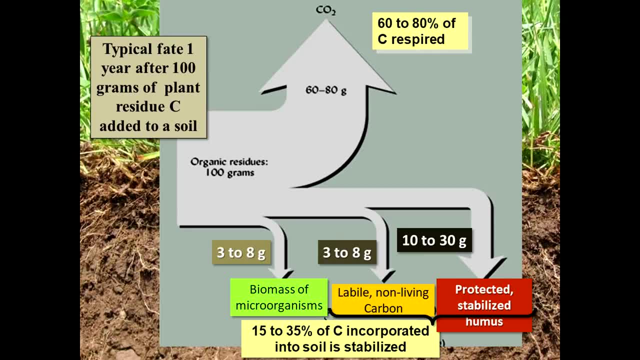 But this is sort of the range that you can expect. You put 100 grams or 100 pounds of plant material into the soil, you can expect 60% to 80% of that to be respired during the first year. In other words, most of it's going to go. 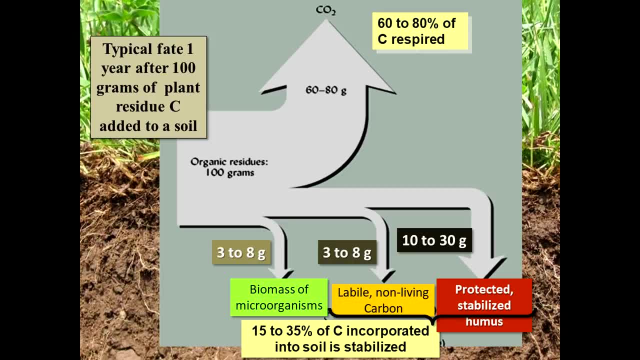 which is good. I mean, that's work. in the process, You can expect to build organic matter in direct relationship to what you're putting in. Most of it's going to get lost. Some of it's going to turn into living organisms. 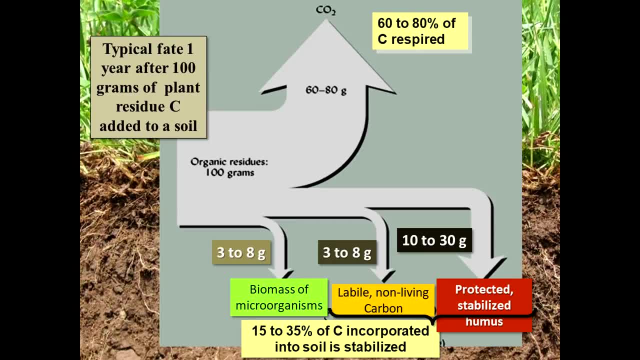 and they're going to be around. You're going to build a biomass- maybe 3% to 8%, pretty similar to what Jennifer was saying, And some of it's going to be various forms of either the remaining plant tissue or the microbes, the dead microbes. 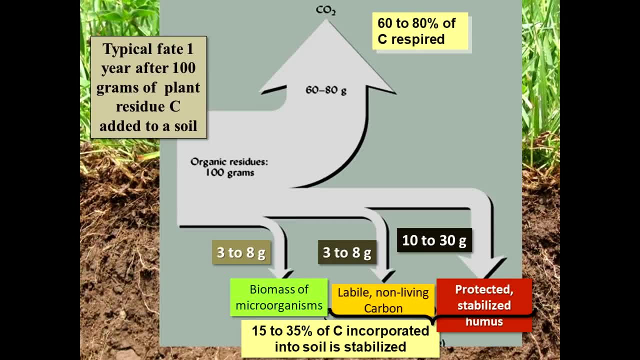 or other forms that have been stabilized. They're going to stay there for a while, And a while might mean decades. It might mean centuries. Sometimes we carbon date this stuff and it stays there for thousands of years. We want some of it to build up. 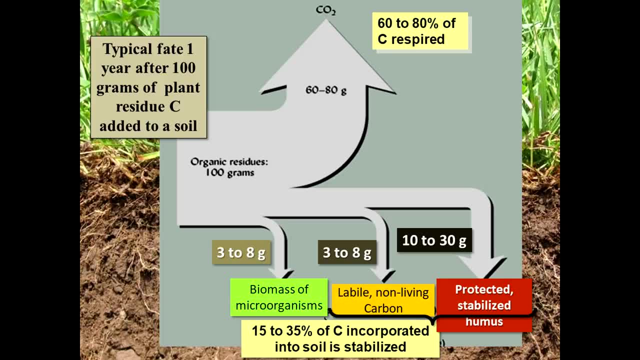 Because, really, when you think about it, microbes and the organisms in the soil are extremely responsive to food. You put a little food on the soil, they take off, They multiply, They turn on their enzymes and they use it up. So why is there any organic matter? 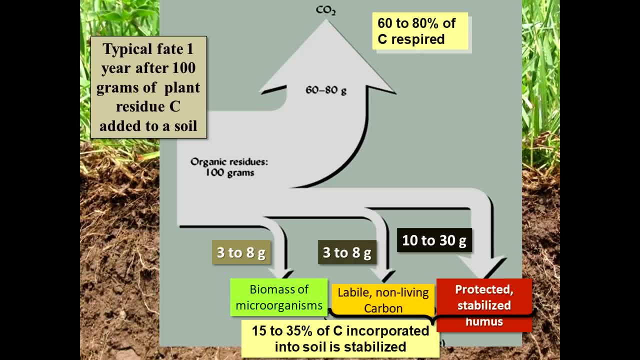 in the soil to begin with, Why doesn't it all get eaten up? There shouldn't be any. Yeah, Because it's not all hamburgers and french fries. It's not all hamburgers and french fries. Well, you're implying that the food 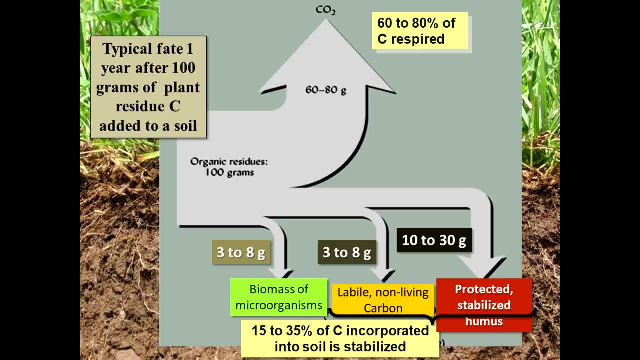 doesn't mean you think there's some cardboard packaging that doesn't get eaten. That's true to some extent, but not much. There are almost any kind of organic food. outside of plastics- Most plastics- there's an organism that can eat it. 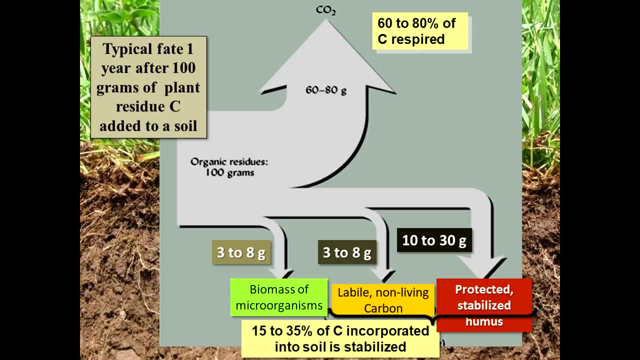 You know the white rot fungi do pretty well on lignin and wood. So biologically you'd think, well, there wouldn't be any soil organic matter. It keeps coming in that you know. if you put in more you're just going to grow more microbes. 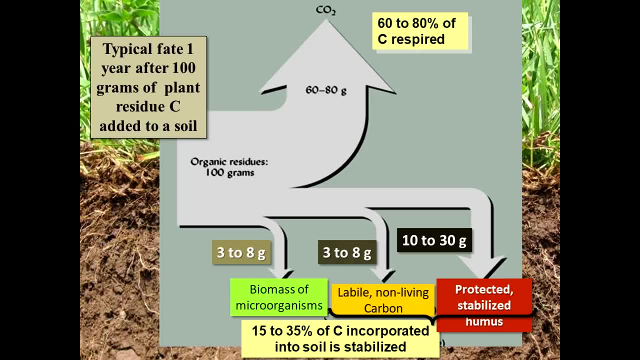 Why doesn't it all get eaten? The reason is that the products of it end up getting into an environment, in the soil, where they can't get digested, where they're either physically protected or they're chemically absorbed onto clay surfaces. It's one of the reasons why clay soils 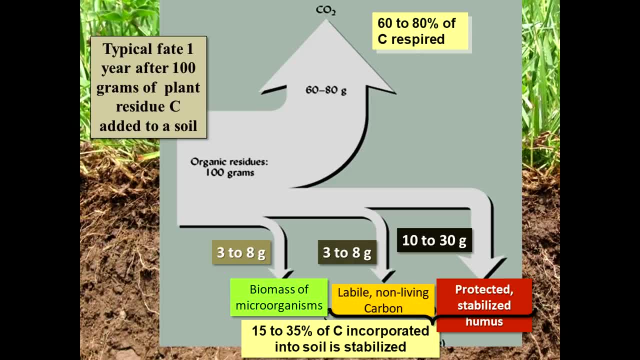 have a lot more organic matter and it's easier to build up than in a sandy soil, Or the environment may be too cold. If things are cold, the whole thing slows down. So if you're in Canada or North Dakota in the same rainfall, 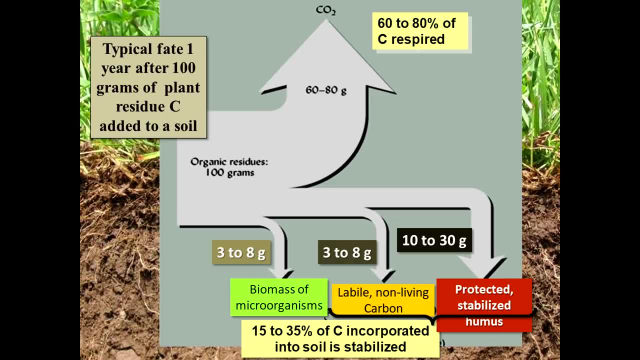 you're going to have a lot more organic matter than in Texas just because it's cold, And the cold slows down the decomposition more than it slows down plant growth, Or it might be too wet. That's why wetlands and low spots and poorly drained soils have more organic matter. 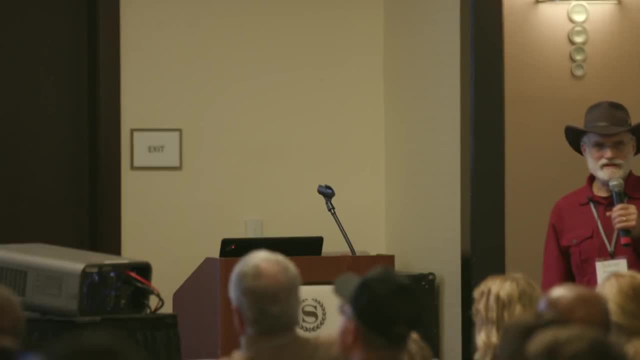 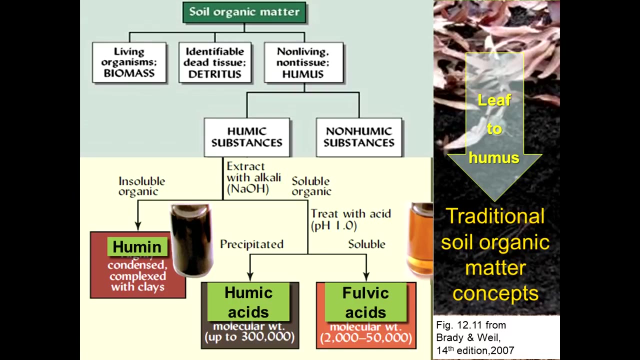 Now we used to think this is a chart from my previous edition of the textbook that I wrote in 2007,, and I was behind the times. For oh, about 150 years scientists have been studying soil organic matter, and they've really missed the boat. 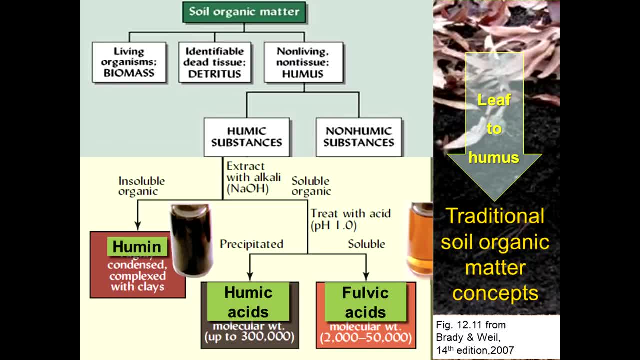 So this might be a little hard on you, but this is sort of a traditional way of defining organic matter. Of course there's the living, there's the dead, and then there's really, really dead. That's Fred Magdoff's terminology. 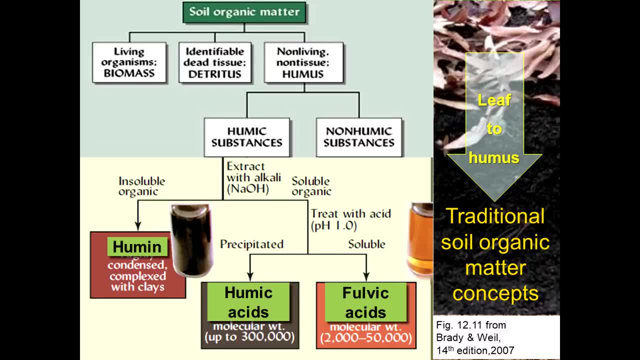 And the really dead is the what we call humus, And we used to think there were these humic substances and non-humic substances. Well, the non-humic substances were things like enzymes and, you know, biomass and stuff like that. 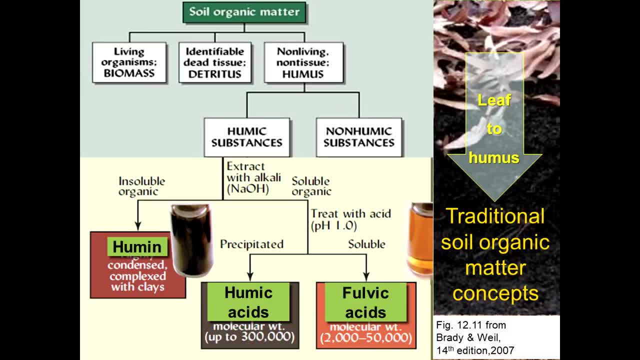 And the humic substances you could extract from the soil, And what they used was sodium hydroxide. So it's been about 150, almost 200 years since they started extracting soil with sodium hydroxide Standard method. Now you use sodium hydroxide around the house. 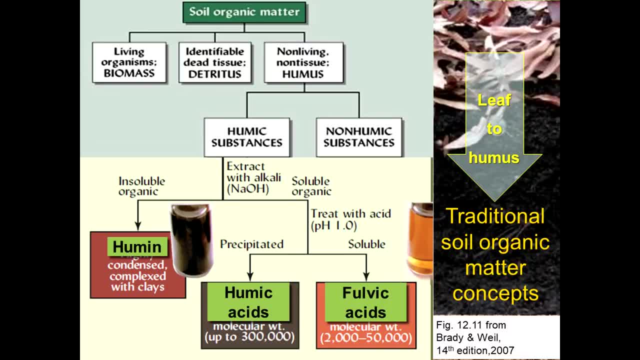 One brand name is Drano right Concentrated sodium hydroxide. And what do you use it for? Put it down the drain to dissolve organic gunk like grease and hair and stuff that's in the drain. right, It does the same thing in the soil. 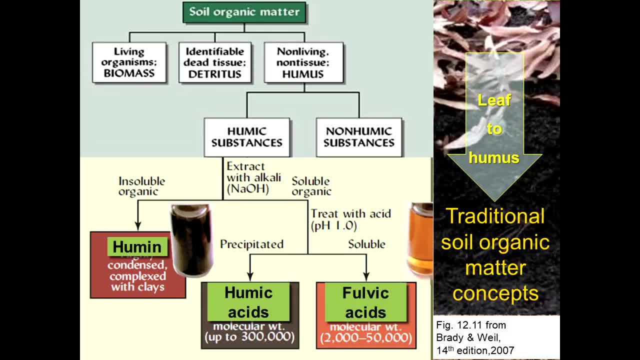 It'll dissolve all the organic matter out of the soil and you'll get this black soup of dissolved organic matter. And almost everything we know about humus has been studied on that black soup that was dissolved out of the soil. Well, it turns out, making that black soup. 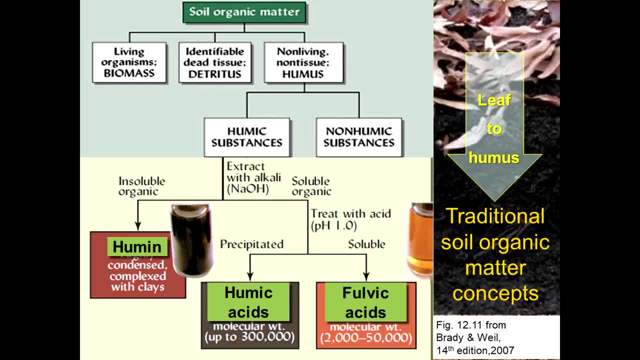 really changed the organic matter, dissolving all that stuff And most of what we thought. oh, it's really a shame There's a humic substances society that's full of scientists that have spent their whole career studying these things in the black soup. 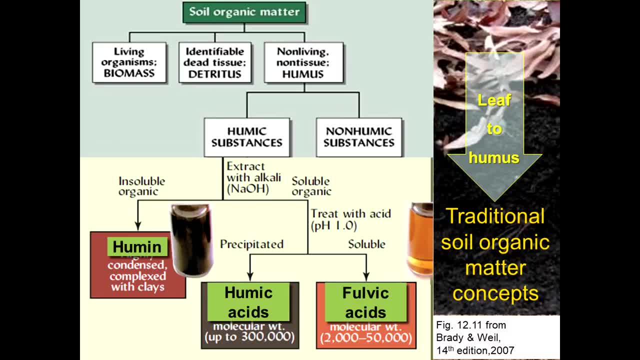 You know this- humic acids and fulvic acids that come out. So the old idea was that leaves would decay and they'd decay longer and they'd be used by the microbes and they'd be turned into bigger and bigger molecules that were so complex that they couldn't decompose. 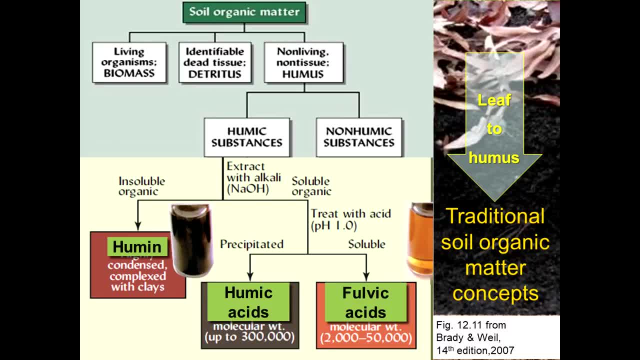 That was kind of the it's not all hamburgers and french fries, I think is what he was probably getting at. But first of all, there's no really chemical reason why complexity would make it harder to decompose. But that's the way people thought about it. 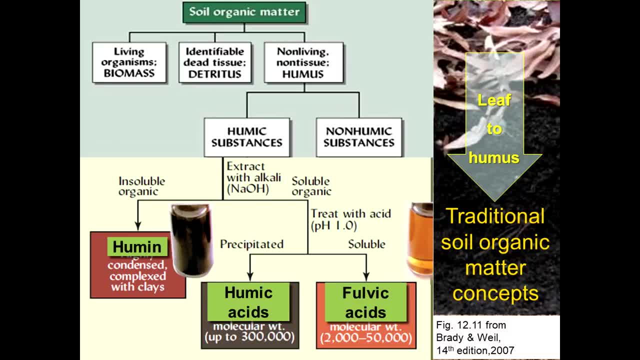 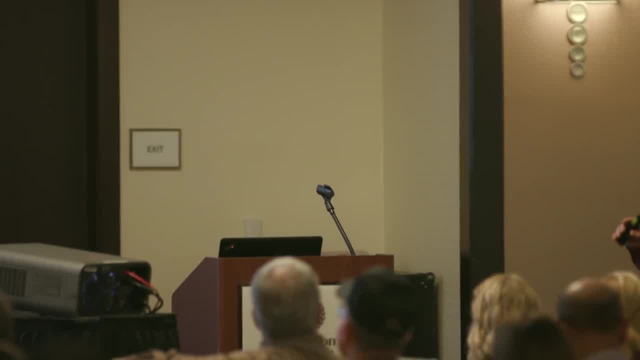 And secondly, it turns out that that's not really what's in the soil. That's what you get in that black soup when you dissolve it in Drano, But when they we now have instrumentation that can look at organic matter in the soil. 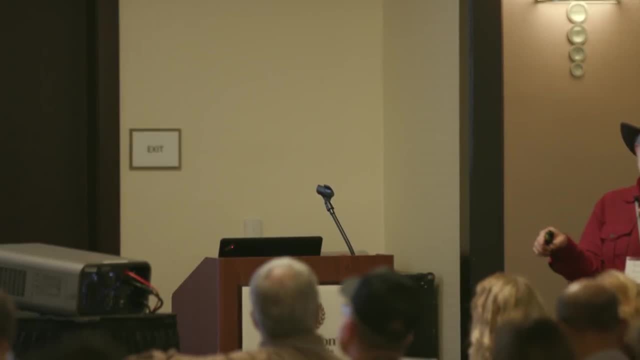 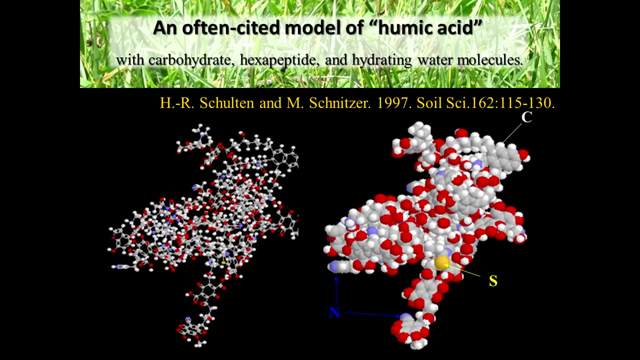 through imaging, through spectroscopy, through there's a number of MRI and exanes. We have a lot of high-tech kinds of instrumentations that can look at the kinds of chemical bonds that are in the soil and the kinds of molecules that are there. 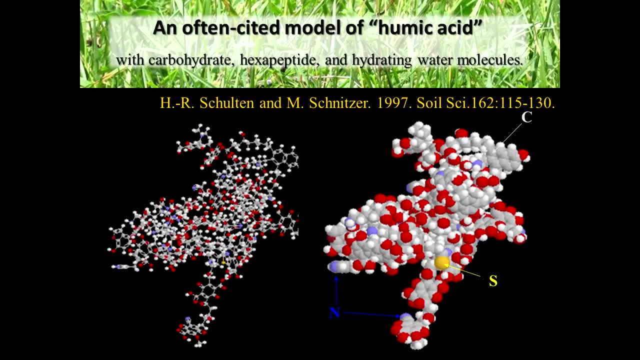 And we don't find this stuff. We don't find these huge, complex molecules. So this is what we used to think humus was made out of. And bless their hearts. children Schnitzer spent their whole career trying to figure out the structure of these molecules. 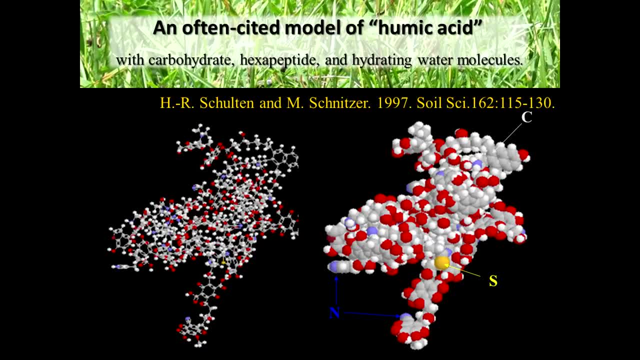 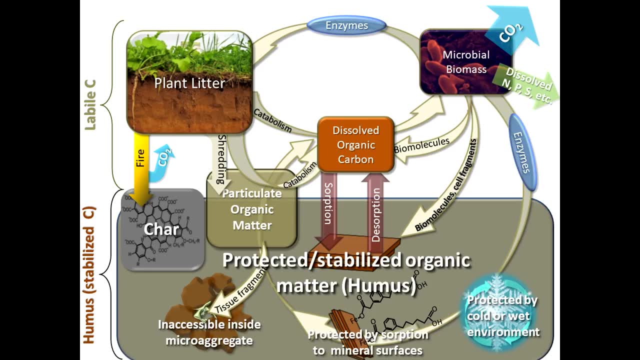 But it was all what's in the black soup. This is what we think is really happening in soil. So this is the diagram for the new edition of my textbook. It came out last year. I think I should have brought a whole box of these. 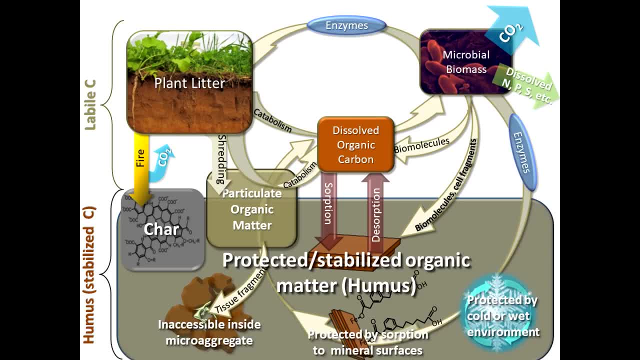 because I'd been asked for them but I didn't. They're online. So organic matter, as I said, starts with plant material And there's a nice cover crop profile of a mixed cover crop, Plant material and microbes. Okay, 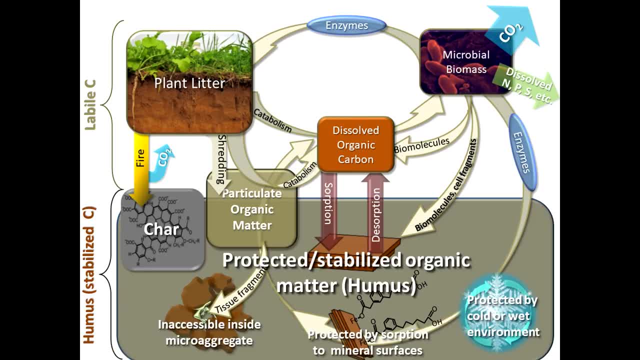 So microbes take this: whatever the plant is giving the dead leaves, the dead roots, the root exudates And most of the microbial digestion takes place outside of the microbial cell. They exude enzymes, exoenzymes, And this breaks down this plant material. 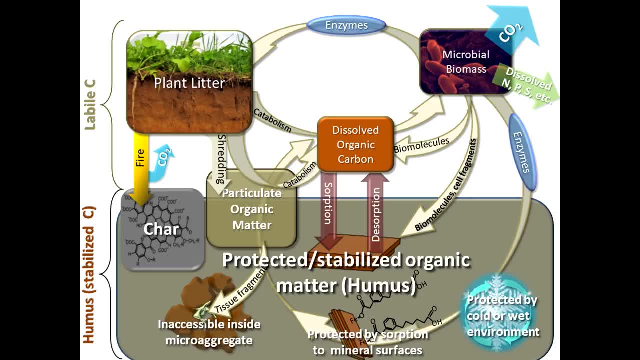 It creates these small dissolved molecules. So we have a lot of dissolved organic carbon And that's what the microbes can take up: the sugars, the amino acids, things like that. Okay, So it's kind of a cycle Now to help this thing out. 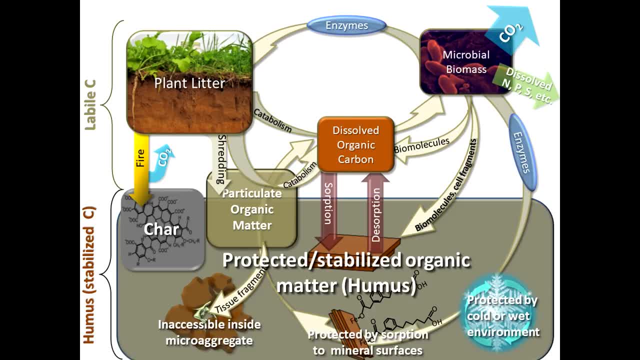 these little critters that Jennifer was talking about, the soil animals, the earthworms, the smaller critters like the columbula and the mites, even some of the nematodes. they can do some shredding, So the bacteria don't have any teeth. 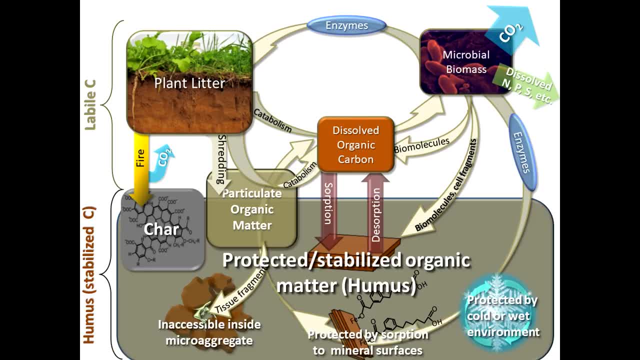 Even the fungi don't have teeth. It's kind of hard to grind up a leaf and get through the coatings and stuff, So that becomes these little bits of plant tissue in the soil. I've got this unlabeled box at the bottom. I'll get to that in a minute. 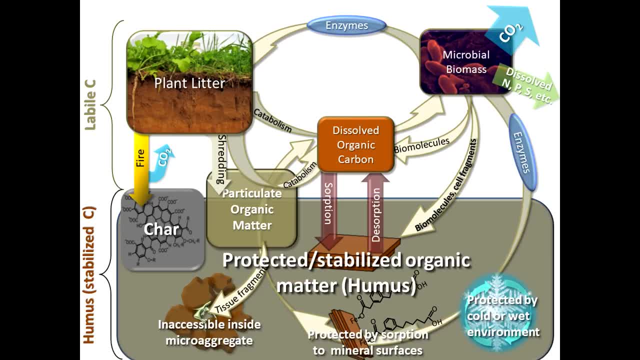 But the soil is full of these tiny little bits of plant tissue called a particulate organic matter, And some of that gets digested with those microbial enzymes, And then the microbes, of course, are producing molecules, including their own cells. So the microbes are growing on this. 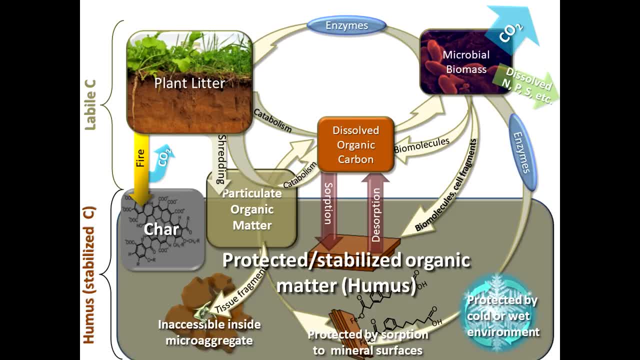 and they're using anywhere from 20 to 30 or 40 percent of the carbon to grow on. Fungi are more efficient than bacteria. Some bacteria are more efficient than others And all the time they're breathing So a lot of this carbon, as we said. 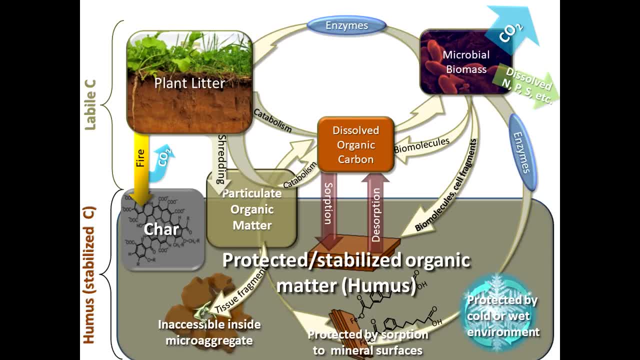 is going up back into the atmosphere And fortunately they're also releasing nutrients from this And this organic, this dulled organic material is being absorbed, especially onto clay surfaces. Clay surfaces will hold these and that will prevent it from being decomposed. 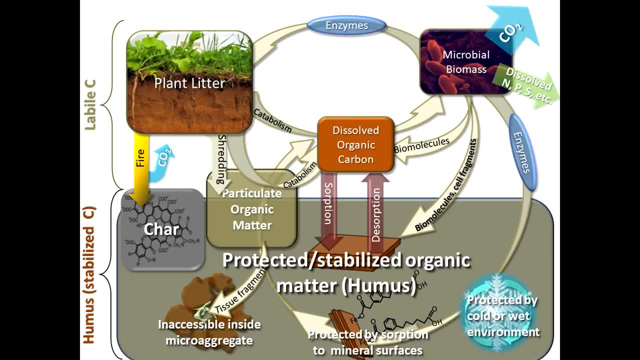 And it will also be desorbed. so it's in equilibrium And the microbial biomass is producing all kinds of microbial compounds and especially cells. So they grow and then they die, And often the cell walls, that is, the debris from the microbes. 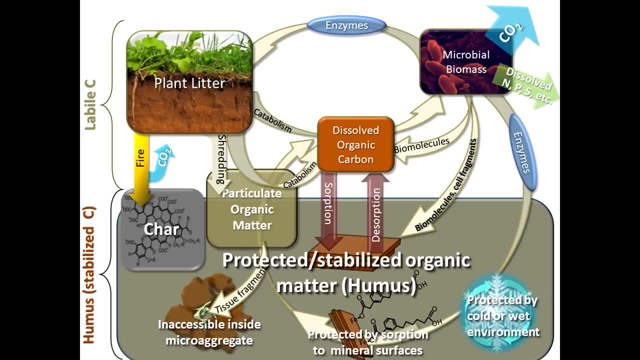 it's no longer plant tissue, but they're little. they're all these tiny cells that are coating the soil particles. When they get absorbed, the insides of the cells will leak out and decompose and release nutrients, But those cell walls will remain there. 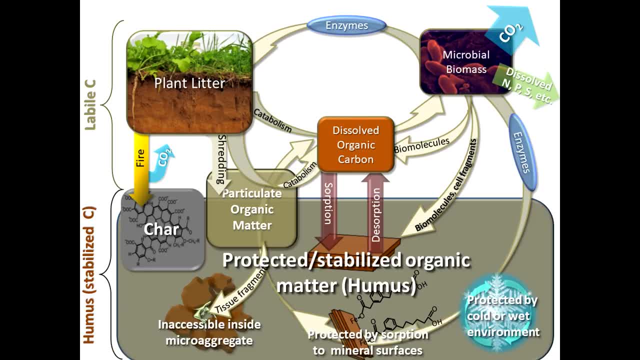 and be kind of fossilized on the surface, And a lot of the organic matter that builds up is actually these cell walls that are tightly absorbed to clay surfaces And, of course, during this process, when there are more nutrients than the microbes need to build their cells. 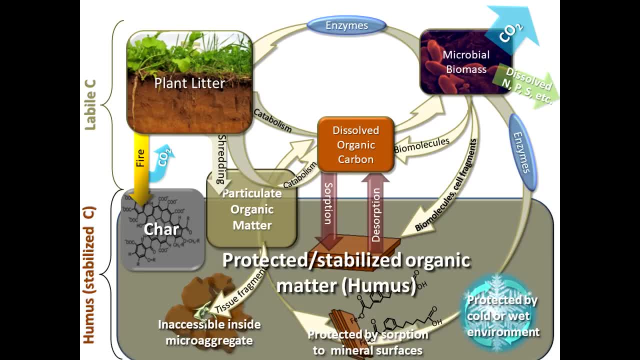 they then excrete these into the solution And that's really promoted, as Jennifer also mentioned. I don't know if you caught that, but those nematodes are really important in keeping the bacteria from growing really big colonies and just holding onto all the nutrients. 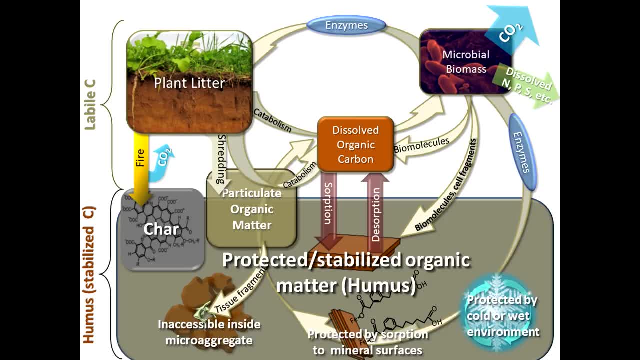 The grazing: you know how grass gets stimulated when you graze it. The regrowth: it's pretty much what happens to the microbial colonies on these soil surfaces. These critters, like the mites and the nematodes, come along and they graze these colonies. 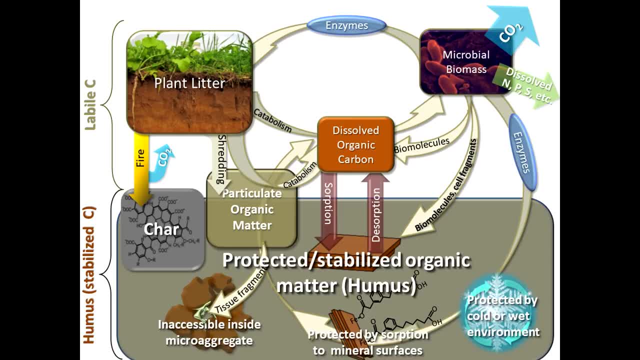 and that stimulates the growth, but it also stimulates the release of nutrients. So as they graze it, they become excess nutrients and they get excreted. And that's what plants are going to use. They're going to use these excess nutrients. 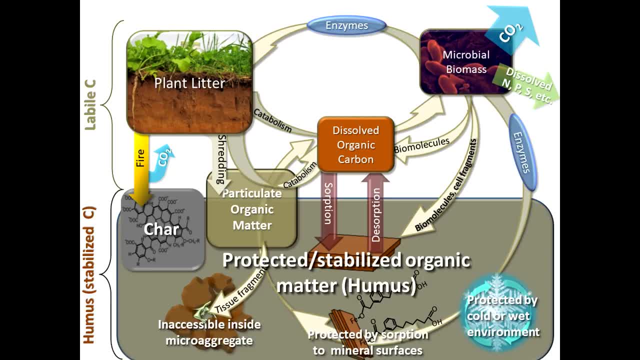 Now there's another interesting wrinkle that we ignored for a long, long time, and that's the product of fire. Fire is a natural part of almost any ecosystem over the millennia. There are prairie fires, there are forest fires. It's a natural phenomenon. 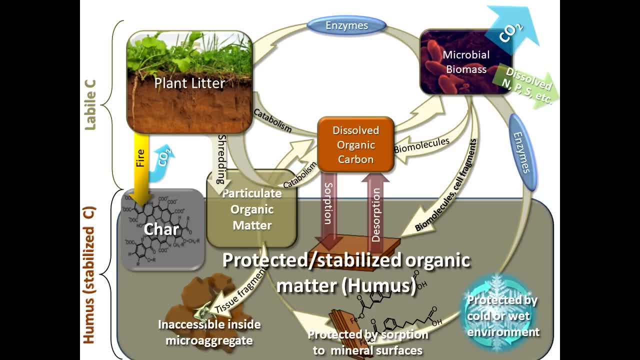 as we well know, if you're from California, right, And for the longest time we just ignored it, because most of the chemical methods we use to measure organic matter. if any of you have heard of the Walkley-Black method, it's from the 1930s. 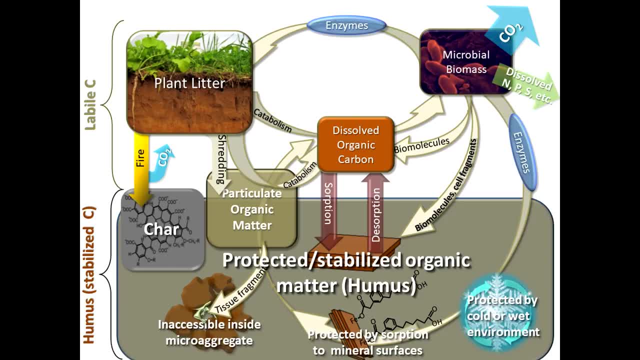 it didn't react with this stuff. Charcoal is very resistant to being oxidized, So they just ignored it. It just didn't count. They had a fudge factor. If you've ever done this, there's sort of a number you multiplied by. 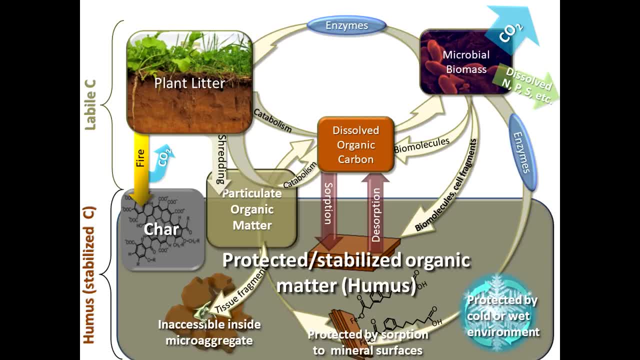 that was supposed to account for this, but it really really didn't. We're now looking at soils and realizing this black carbon is really important. It's very stable. It's very stable for the most part. It has a tremendous amount of surface area. 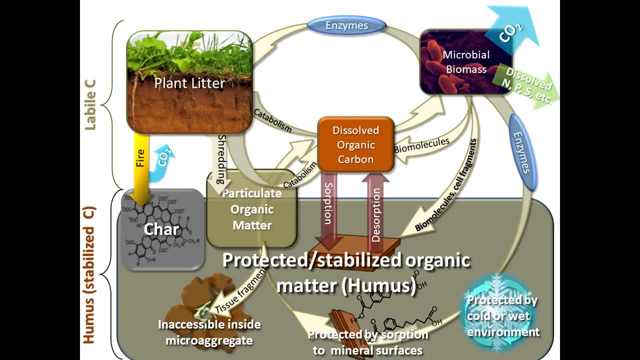 You've heard of biochar. That's where we intentionally make this stuff as a soil amendment. But soils have a lot of this black carbon in it. It's not ash, It's from the low oxygen burning right that produces char. 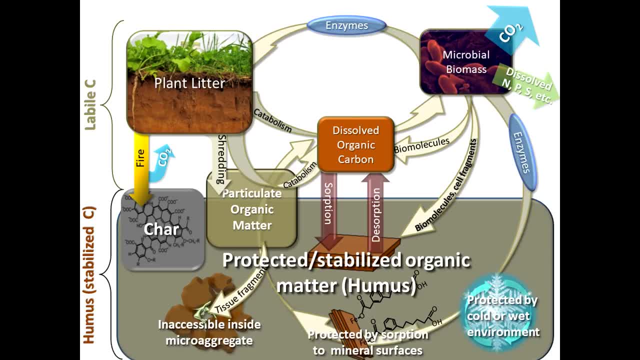 And then that's very stable. So a lot of what we, a lot of the properties we ascribe to these mythical humic substances, actually are being probably due to some of this black carbon in soils, especially the grassland, prairie soils, the mollusols. 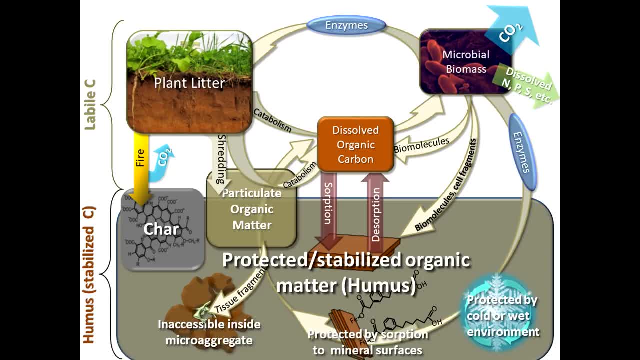 that have a lot of black carbon in them. Now why does it accumulate? Because of conditions in the soil, not so much the chemistry. Most of these are molecules that we can recognize. They're proteins, They're plant molecules, They're microbial molecules. 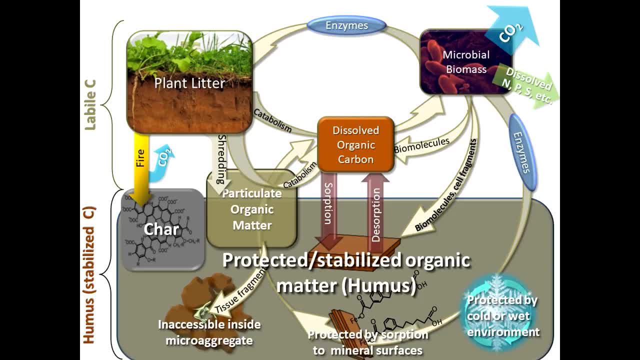 They're components of cell walls, But they're protected because of the environment. They may be too cold or too wet, either in the whole soil or in micro-sites in the soil, Or they're absorbed through metals, So these biomolecules get absorbed onto the clay surface. 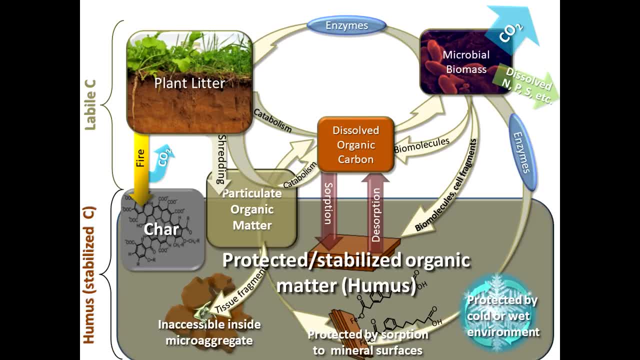 usually from a metal like calcium or an iron bond, And then the enzymes that normally would break them down can't get to the reactive sites, and so then they accumulate, And that's one of the main reasons why having clay in the soil or even silt to some degree, 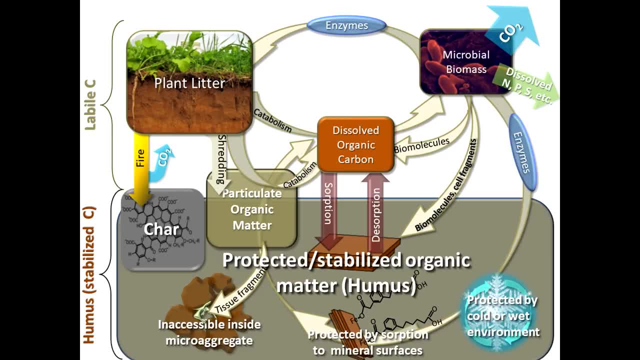 will enhance the accumulation of organic matter because it puts some of this stuff away. It's like taking some of the food and putting it in the freezer where it's not going to, like putting the ice cream in the freezer where it won't melt, I guess. 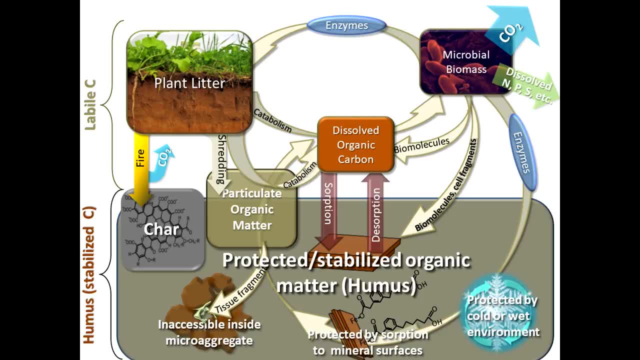 Now this particular organic matter is free to decompose if it's exposed, But aggregates tend to build up around it. So you get through the process of bacteria and through fungi. They're bringing soil particles together and entrapping little bits of this relatively undecomposed. 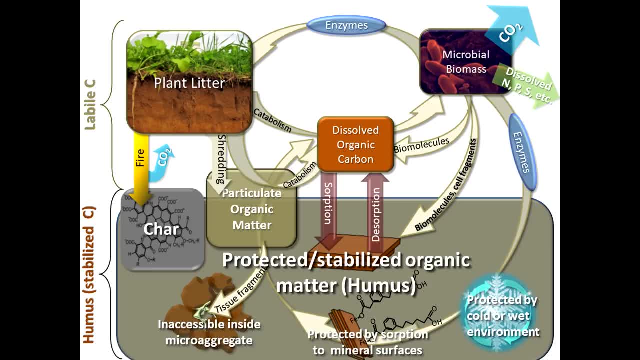 mostly plant material, also some microbial cells. So this is responsible for protecting and building up organic matter by physically occluding it inside these really small pores where even the bacteria can't get at it, And of course tillage breaks that up. So this is a real important reason. 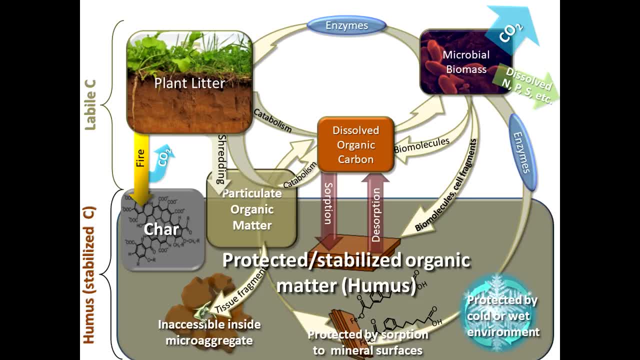 why aggregation is so important, And we're talking about micro aggregates- not, they're almost too small to see, But it's the difference between a dispersed soil and an aggregated soil. So these are all conditions that help protect that, And this results in some of the organic matter being 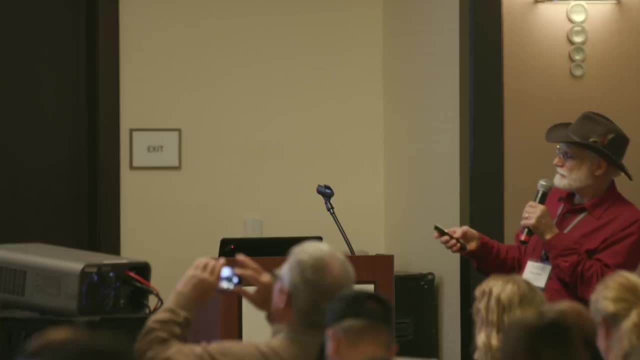 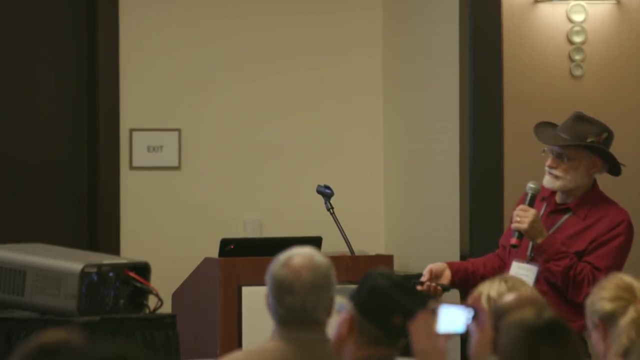 whoop too quick on the trigger here. huh, Some of the organic matter being labile or active turning over being eaten up. it's fuel, it's readily decomposable And some of it becoming stabilized- And I still like to use the word humus. 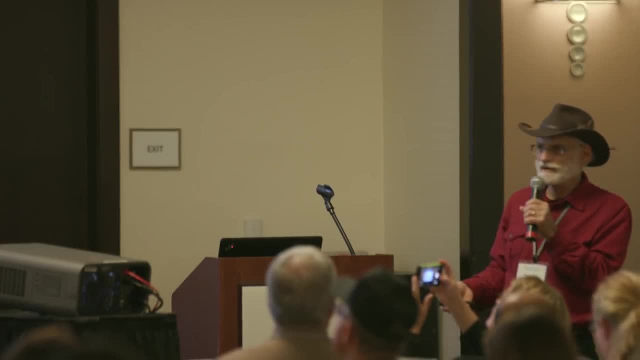 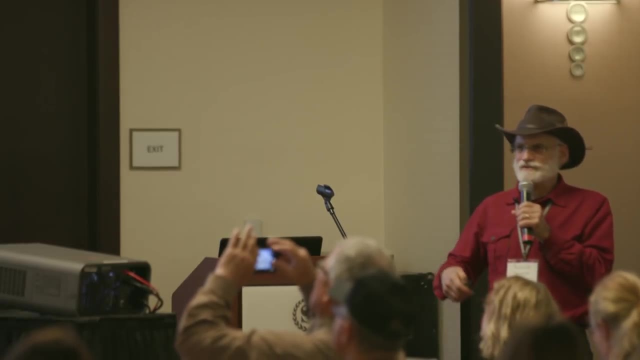 because we know what it is. It just turns out to be something different than we thought, But it's the stable organic matter that builds up in the soil. Both of them have a function. There's cash flow up here and there's capital down there. 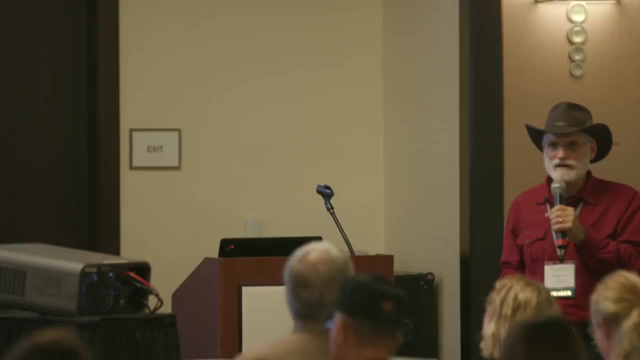 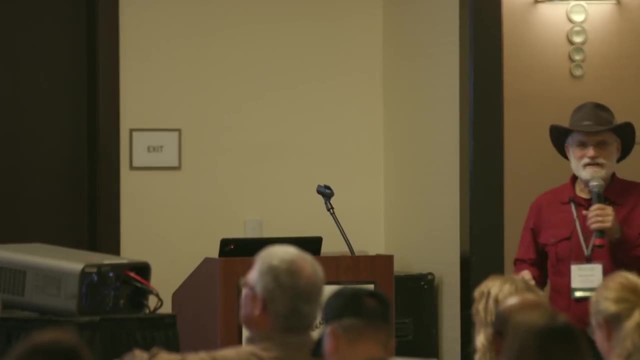 And you need to maintain both, And the only way you can maintain both is to have a good income. right, And that's what we need to have is a good income so we can spend some These aggregates, these are things. if you take some soil next time you're out. 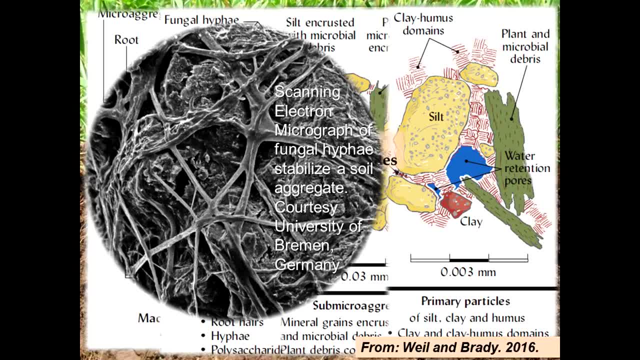 out of the hotel, wherever you are, some of your own soil and take a little bit of it and crumble it down. this is one of the psychologically most satisfying things you can do anyway, right? Especially if you're a no-tiller. 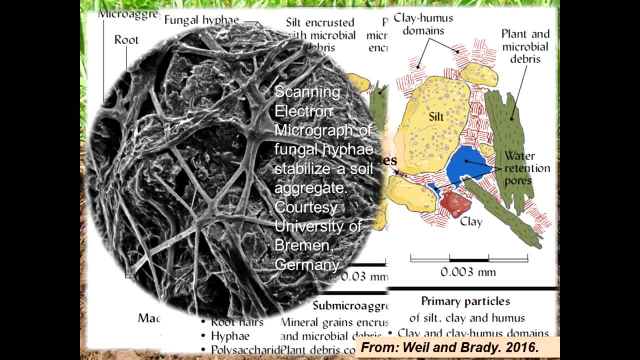 You dig up a chunk of your soil and you get a handful of this when it's about the right moisture and you start crumbling it And just the way it sort of crumbles and falls apart into these natural aggregates is just a very satisfying feeling. 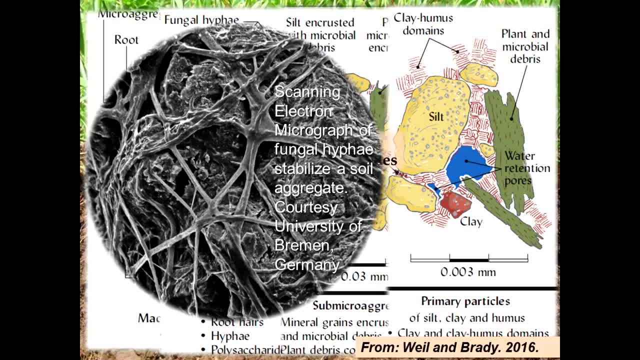 It's not sticky, It's not gooey, It's just crumbly. And you do that, and then you look for the smallest little particles that you can find, Put them on your finger And you think I found a particle. 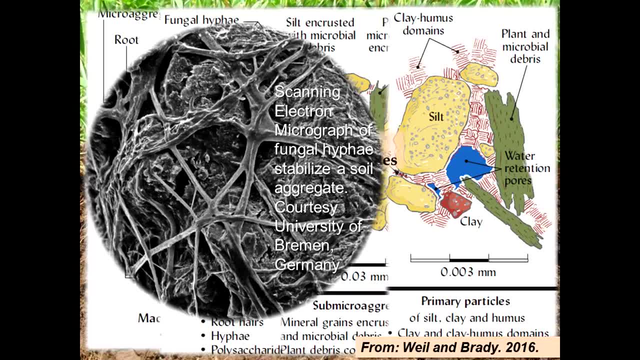 I could get rich doing this if you're willing to bet against me. I bet that if you take that smallest little particle you can find and you rub it, it's going to turn out not to be a particle, It's going to turn out to be an aggregate. 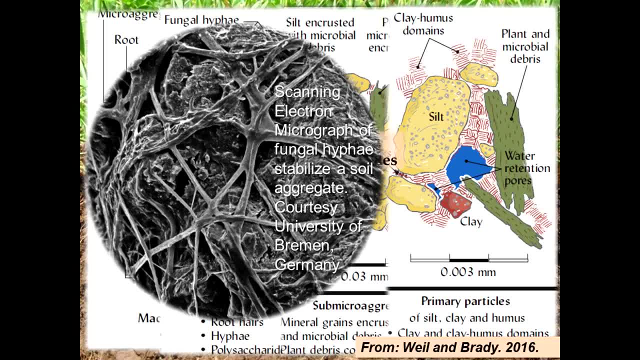 of a thousand particles, Even the smallest ones. So those little, tiny particles that are almost too small to see are really clumps and aggregates and that's where the organic matter is hiding And that's what makes the soil function. So we see these big ones. 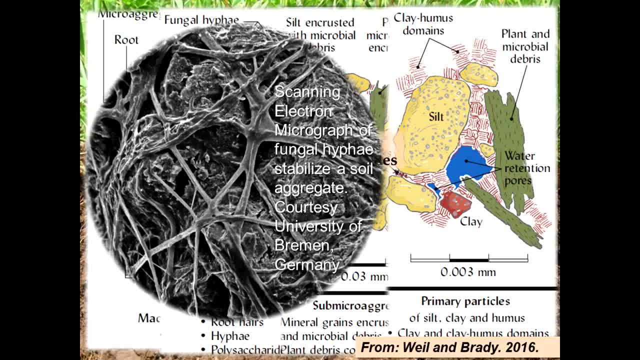 that are several millimeters across, maybe a quarter of an inch. Those are nice big aggregates that are held together by roots, But they're made up of these smaller aggregates, So we take a look at a smaller one. That's where the fungal hyphae really become important. 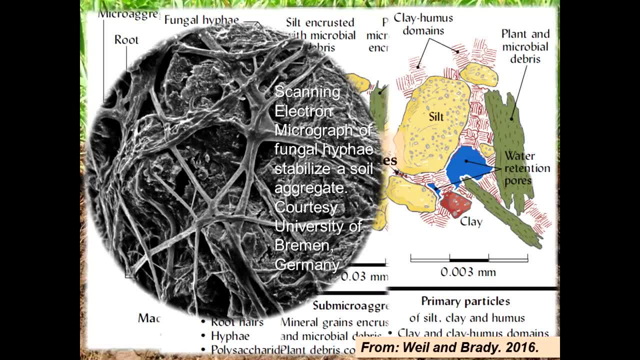 Gluing these together. these green things are the fungal hyphae. Here's your plant root. But even those are made up of even smaller aggregates, So it's a hierarchical structure. So this is a scanning electron microscope from the University of Bremen. 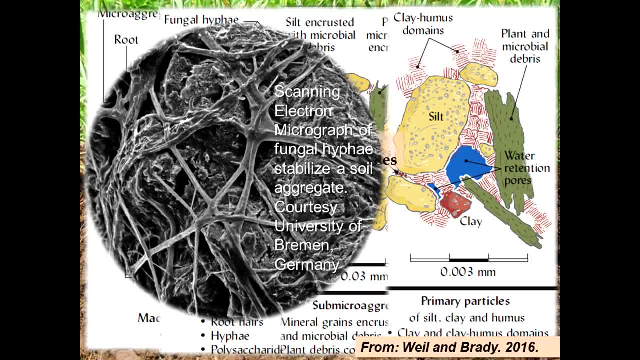 that shows how these aggregates are just covered with a net of hyphae. This is really the sort of hair net that's holding the soil together. The tillage disrupts and not feeding organic. These are living, They are eating, They have to have organic matter. 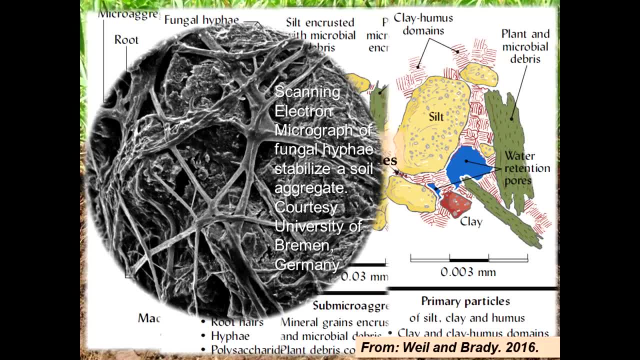 to keep them going. And then at the really micro side, the first day scale, you can see these little bits of particulate organic matter and these little clay particles holding it together. And then down here you can see that the clay at the very smallest scale. 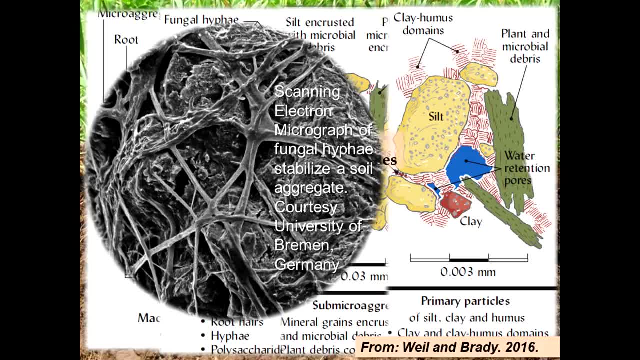 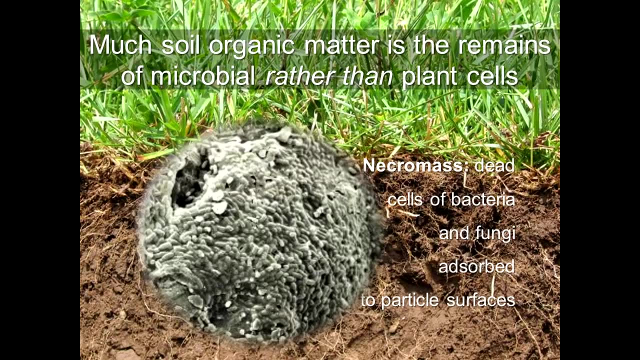 the clay has an important function of holding these particles together as well, And remember that these little tiny pores are where the water is for your plants. So one of these insights that I mentioned that may have slipped by you is that we used to think of all this organic matter. 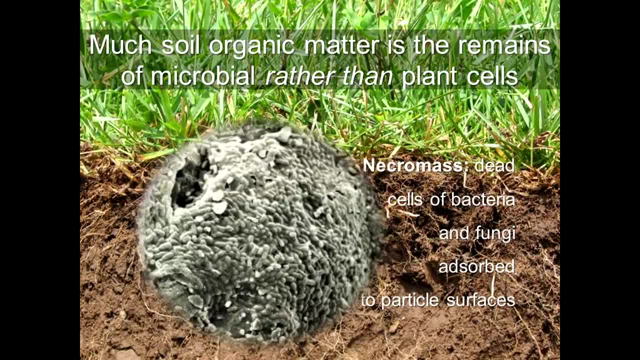 as being of plant origin, But, as Jennifer said, we're now finding that a lot of it is actually dead bacterial archaea. Does anybody know what archaea are? It's another thing that's changed, and some of us went to high school and learned biology. 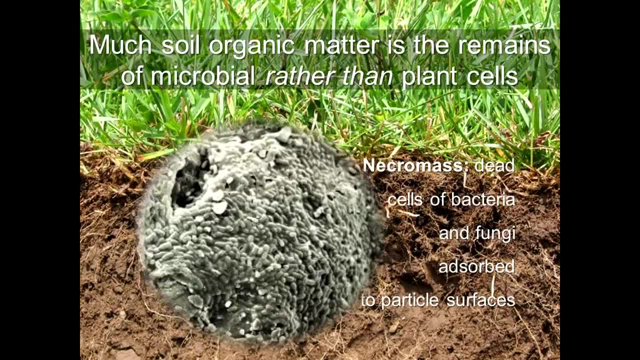 I never learned about archaea when I was in high school. In fact, I don't think I learned about them in college either. So archaea are a whole other brand of life. They're basically three branches of life on this planet. The bacteria are one of them. 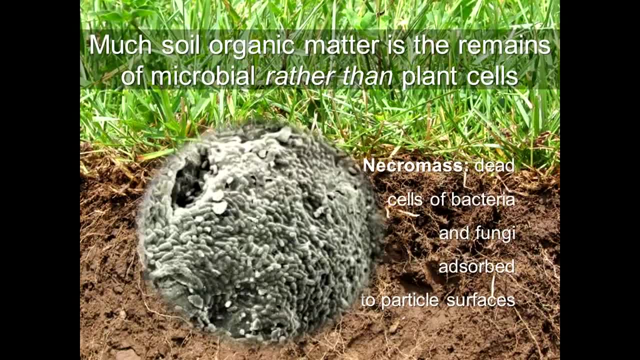 The archaea are another. Everything else is like us or in the eukaryotes, So you are more closely related to a mushroom or a fungal hyphae than the bacteria are related to the archaea, even though they look pretty similar under the microscope. 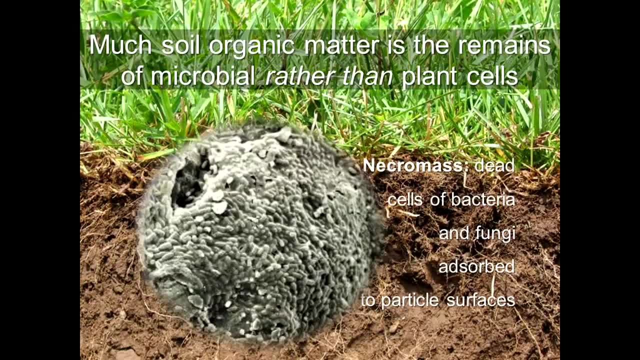 So there are all these cells and not all of them decompose. The cell walls are pretty resistant. They get absorbed. So you have all these sort of absorbed dead cells that are an important part of the organic matter. It's how we store carbon and nutrients. 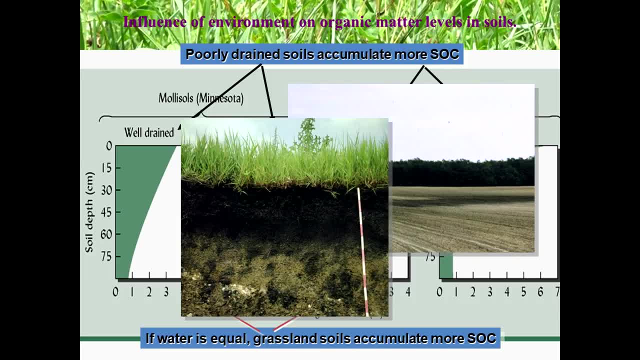 And then, as we said, the conditions. you have to be realistic as to what you can do with organic matter and building it. A lot of it is based on the conditions you have on your farm and where you are. This is just an example. 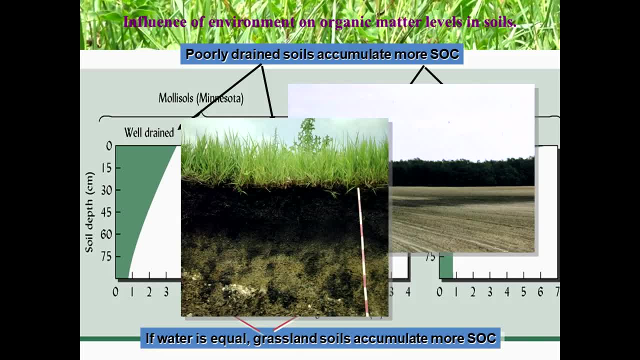 If you've got the mollusols, grassland soils in Minnesota, they're going to have more organic matter than forested soils in Indiana will. And if they're poorly drained, that is, they're wetter, they're going to have more organic matter. 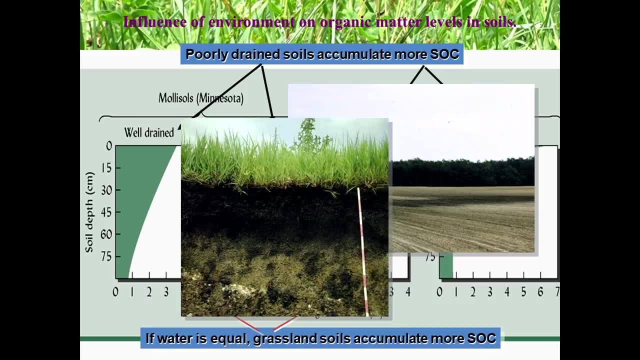 than if they're at the top of the hill and they're well drained, because less oxygen means it's going to decompose, and that's going to be true in forested soils and grassland soils, So it doesn't take a lot of topography. 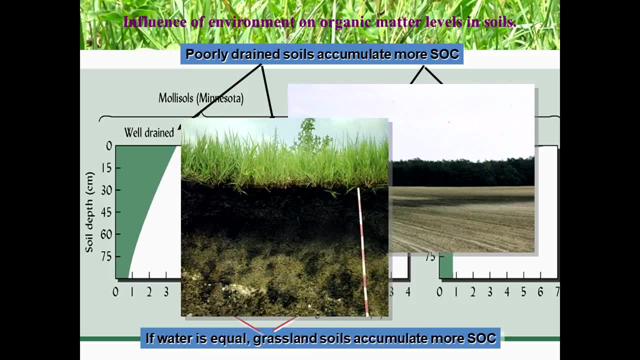 This is on the eastern shore of Maryland. It's pretty flat, but you get a little bit lower and you can see much darker soil. That's a tilled field. That's about. the only good thing about tillage is that you can see the changes in soil color. 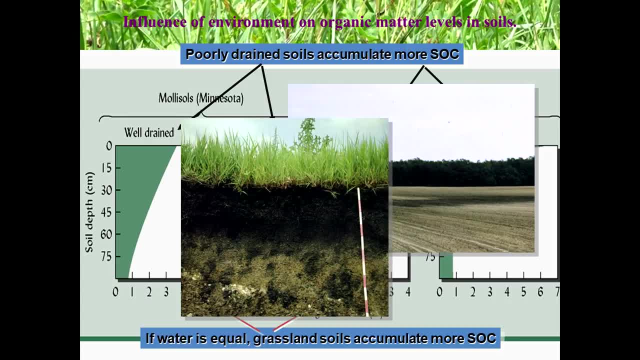 So this is an old picture, back when they used to till in Maryland. You know very few farmers till in Maryland anymore on the eastern shore And you can know, of course, that the kind of ecosystem that was there before you started your farm. 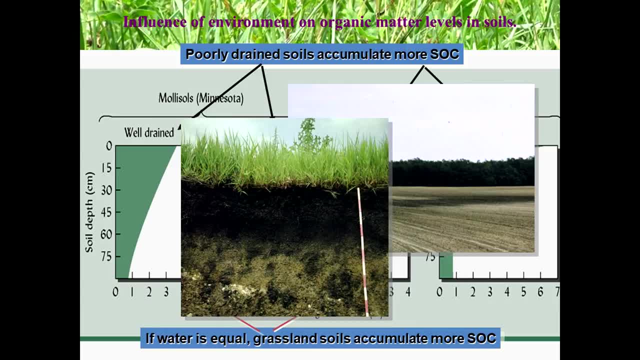 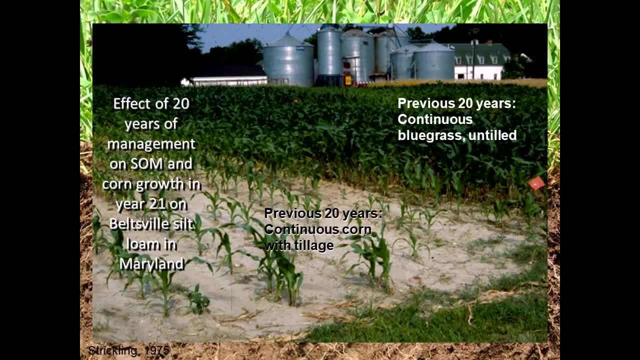 has a big impact on how much organic matter you're going to build up. I might skip through this. This was an old experiment that was done in Maryland And for 20 years the guy that did this experiment, Ed Strickling. 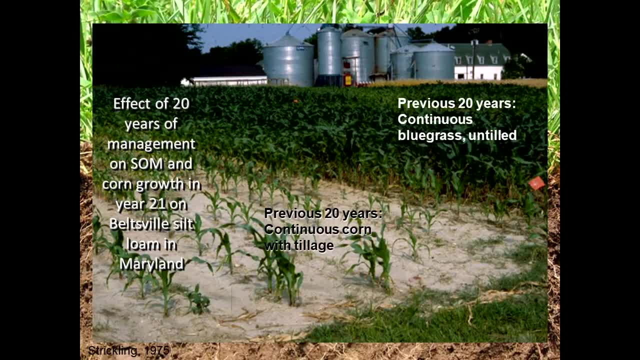 had a couple of different rotations And the extremes were: he planted corn every year with tillage versus. he left the thing in bluegrass sod. It implied the same rates of nitrogen to everything. After 20 years he grew corn on everything. He plowed it up and grew corn on everything. 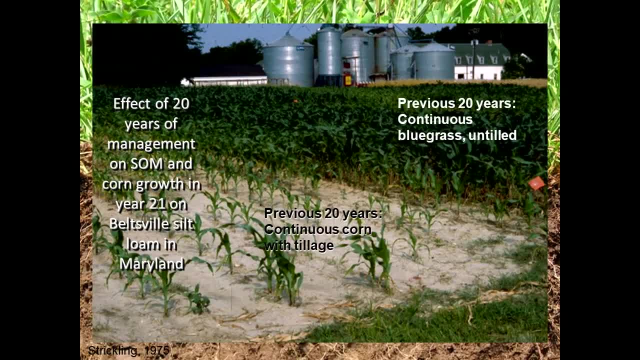 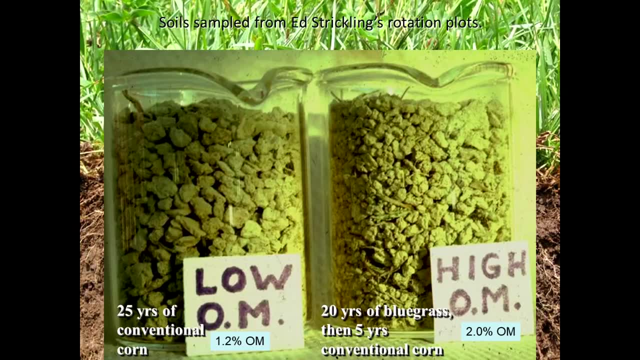 So he was looking at the impact of different kinds of management. He had different rotations And I came in and sampled those in the 25th year of this experiment And the soils look pretty similar. These are silt loams, not particularly well-structured. 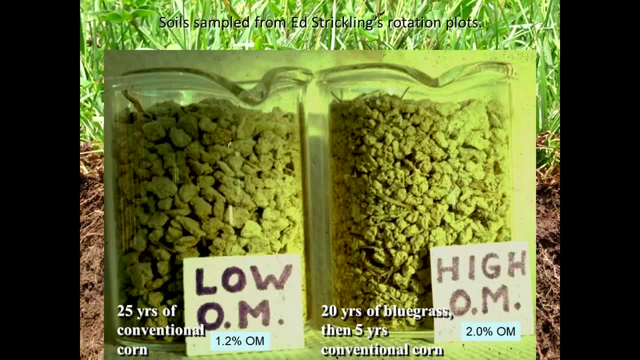 But there was a difference in organic matter that occurred after 20 years of difference in management. Growing corn and tilling it reduced the organic matter a little And growing grass increased it a little. I think it started around 1.5. So there was a difference. 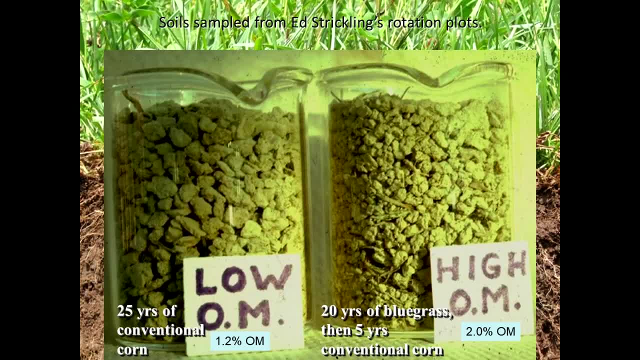 And this is percent organic matter. So percent carbon would be about half that. So fairly small difference, but significant after 20 years. But look what happens when you add water to these beakers. And this is what happens when it rains on your field. 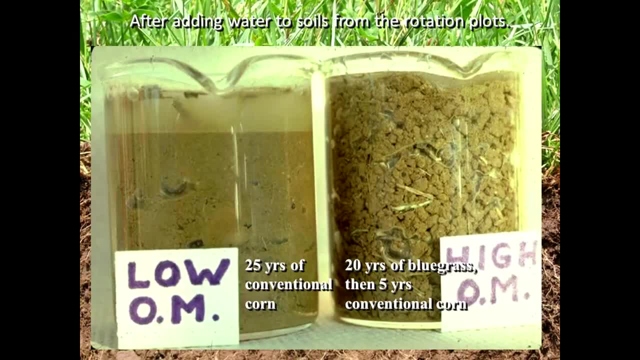 Same amount of water added to each beaker. You've used up the active organic matter that glues those aggregates together by tilling it and not returning much residue and not having perennial vegetation as opposed to maintaining it, And you can see these aggregates just maintained. 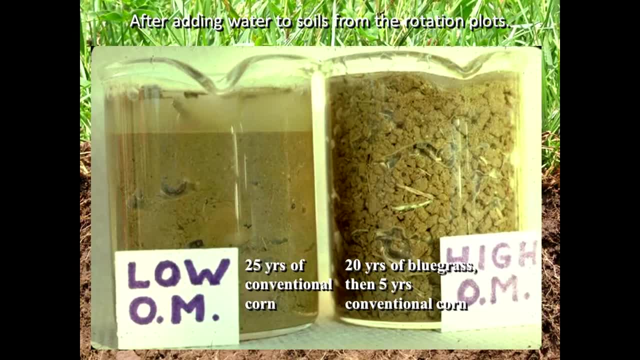 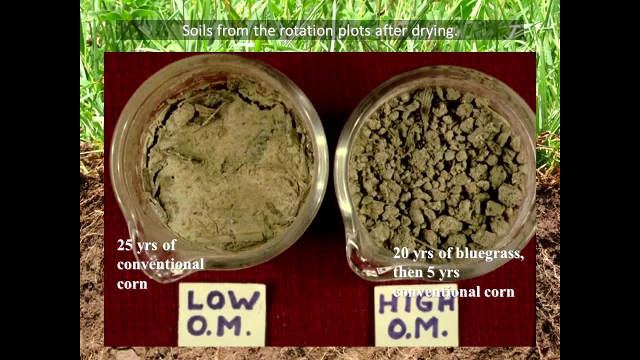 And this is holding all the water, And this one has just settled down and it can't even hold all the water And, of course, when it dries, you see that How many neighbors do you have? I'm sure none of your fields are tilled. 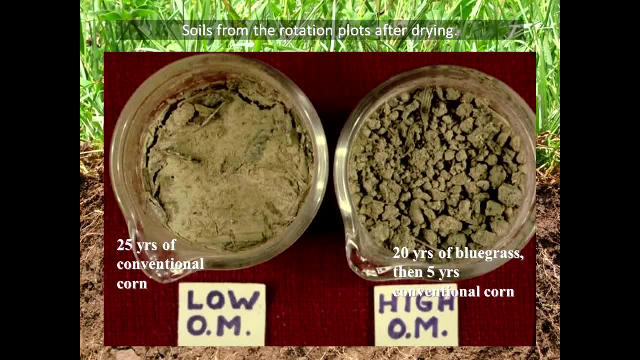 But if you walk out into your neighbor's fields, that's what the surface looks like in the middle of summer, isn't it? That's what most agricultural land in America looks like, especially out in California, Just to bother Jennifer, who works out there now: 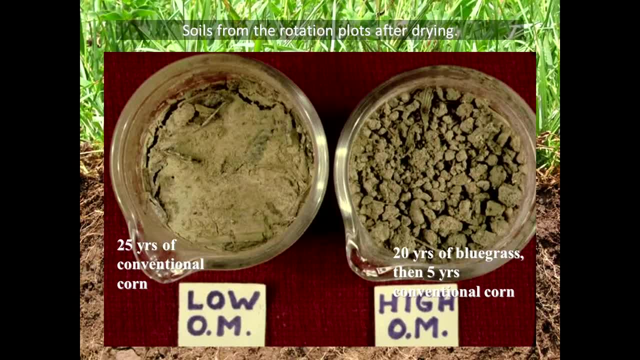 California. every time I visit California I think, oh, there's our problem child. How do we solve their problems in their economic environment so that they can do some of this stuff? And I know there are farmers out there that are doing it. 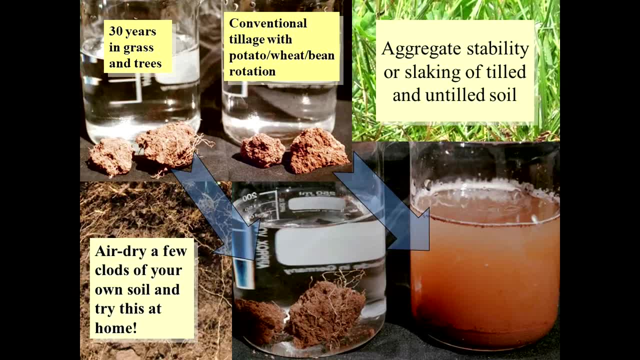 So this is something you can take home and do. Do this with your fields. Dig up a few little clods, Let them dry on the kitchen table for a few days and then drop them in a glass of water, And you can score yourself. 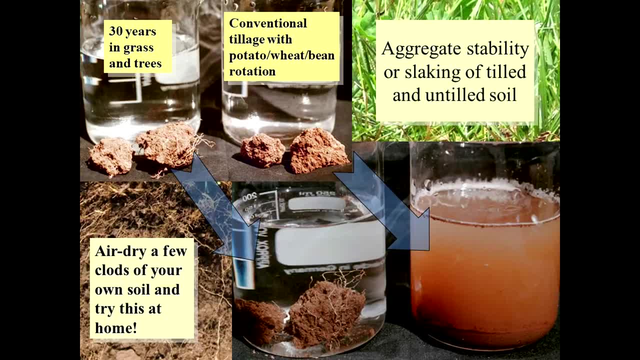 as to how well you're doing. This is one of the simplest and most meaningful tests for looking at soil health. Just how does this hold together when it gets wet? This is a soil that's been in permanent vegetation. This is one that's been not well managed. 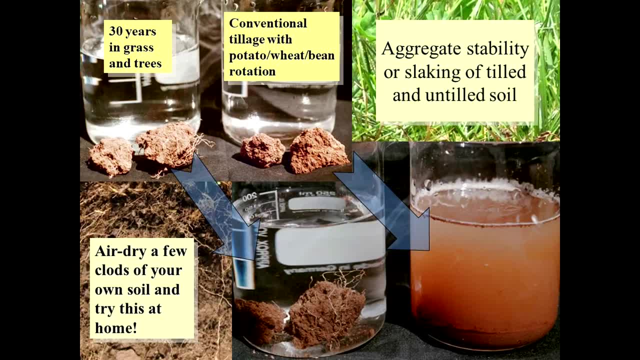 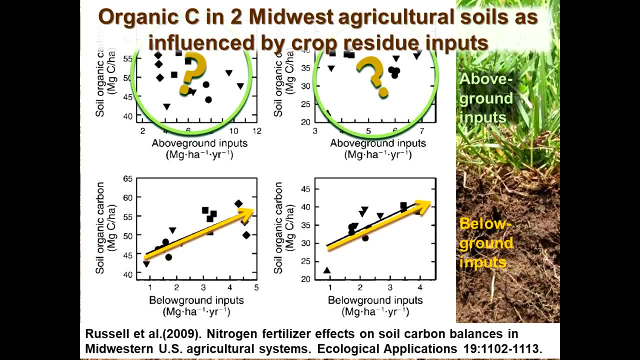 This happens to be from Africa. You can do this anywhere in the world. Do it here in Indiana. you'll get the same thing, I think. do I have time? I don't know When is this, So there's not much time. 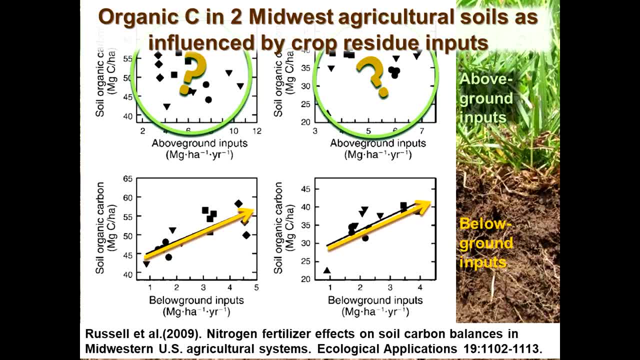 Okay, so I want to talk a little bit about how you can build organic matter through building productive crops, And one of the contraindications and one of the controversial issues is nitrogen fertilizer, because it really is a Goldilocks situation: It grows bigger crops. 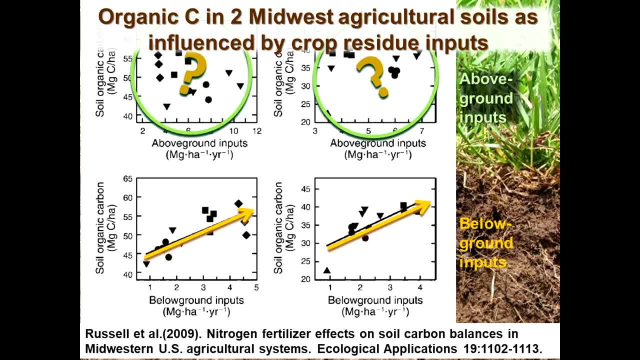 which produces more carbon, but it also speeds decomposition. It reduces the carbon to nitrogen ratio and it also stimulates the decomposition tremendously, So you don't want to have too much of it. aside from the fact that it's wasting money and it pollutes your water. 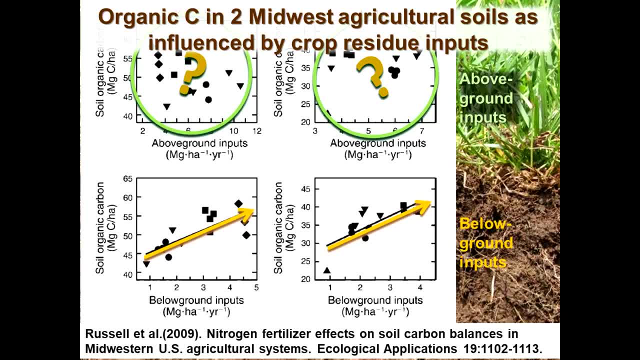 and makes your neighbors in Toledo pretty angry with you, right? And it's really the below ground, organic matter that you want to build up. So this is one thing we've also learned in recent years- is that a pound of roots is worth about a pound and a half. 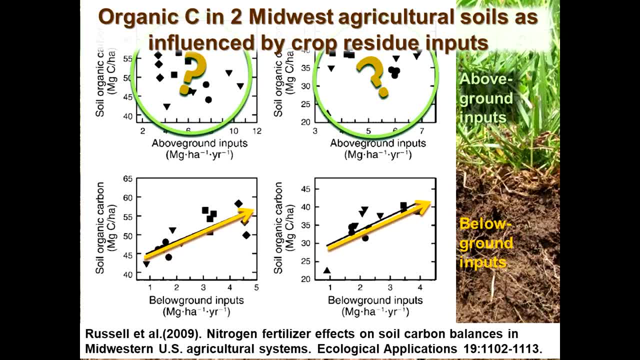 of above ground material in terms of building organic matter. Part of that's because of where the roots are. They don't get added to the top, They get added intimately in the middle of those aggregates, And part of it's what the roots are made out of. 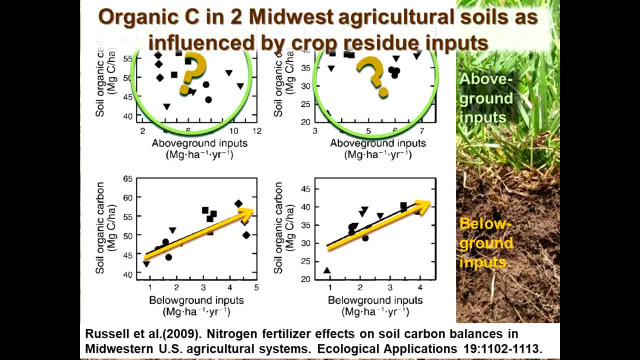 They have a lot of suber in them which decomposes much more slowly and tends to accumulate. What this study showed- and this was looking at a number of sites in the Midwest- was that the relationship between the organic carbon and this is a long term study. 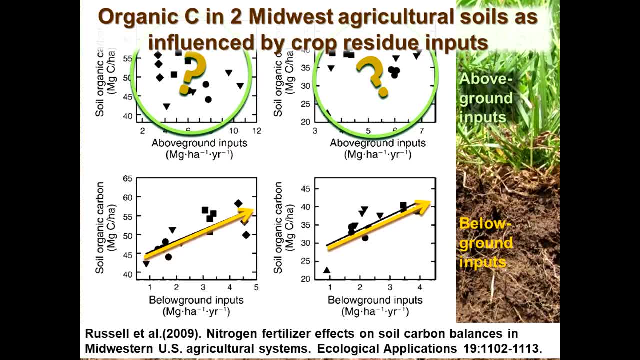 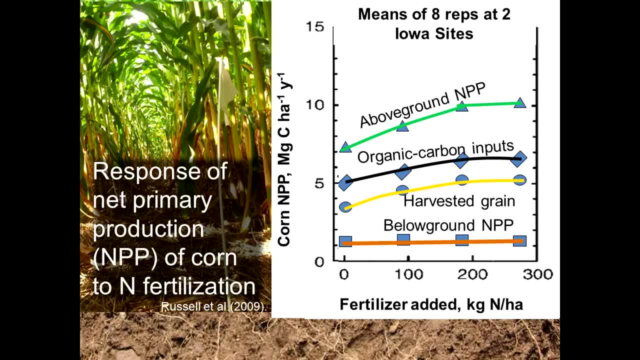 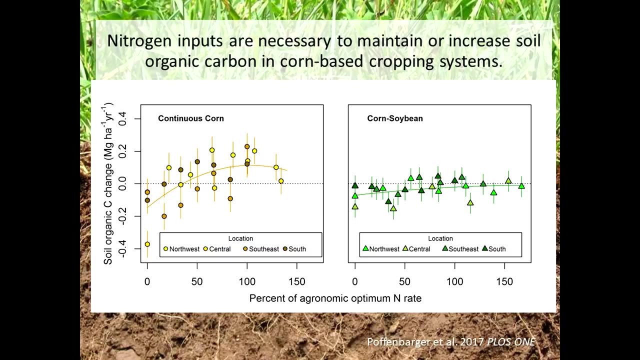 so after many years the organic carbon was related to the below ground inputs much more than to the above ground inputs. Basically, fertilizer doesn't grow roots very well. It stimulates top growth much more than below ground. However, too little nitrogen is also not very smart. 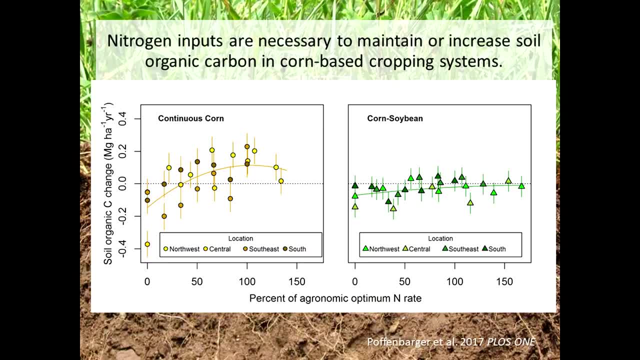 because you don't grow enough plant material to keep up with the soil respiration and you're falling behind. So if you under fertilize, this is also unfortunately none. of this is done on no-till with cover crops. So this is cultivated corn. 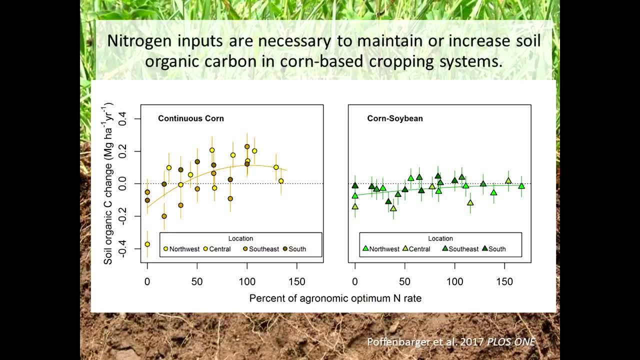 This is a recent paper that looked at studies that went on for several decades in Iowa, But you can see that this is the soil organic matter change from the beginning. The zero would be just holding. still At the lowest fertilizer rates, you were losing carbon. 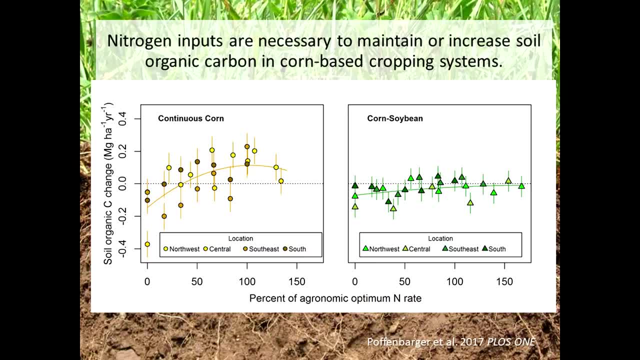 and at the highest you started coming down again to this continuous corn. With soybeans it's harder to maintain organic matter because soybean residue decomposes so easily and there's a lot less of it. So every second year you're putting a lot less carbon in. 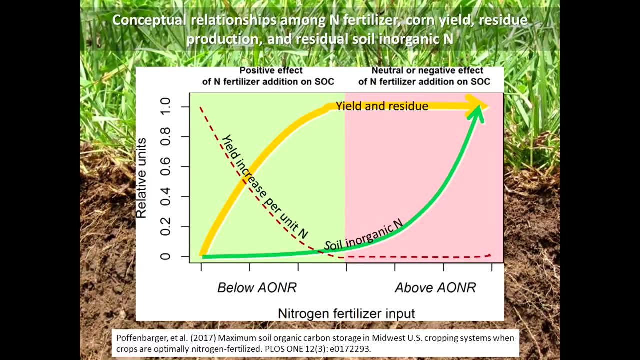 So this is the concept. is that adding nitrogen to the point where it doesn't increase yields anymore economically is a good thing? Adding nitrogen from legumes, adding it from manure, adding it from fertilizer, whatever the source? We don't always have that pinned down very well, right. 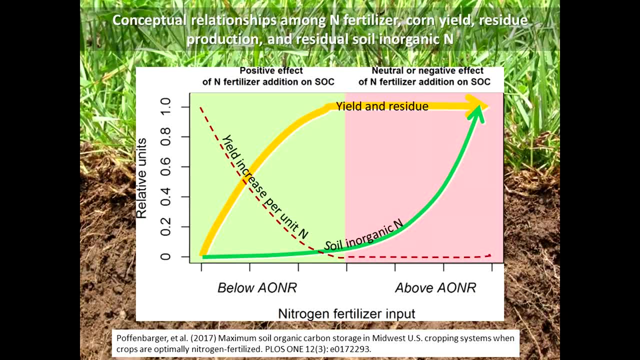 That's one of the issues that's hard to figure out. How much is the right amount of nitrogen? But we need to figure out what that agronomic optimum nitrogen is. We often miscalculate that And how many people fertilize for that one year. 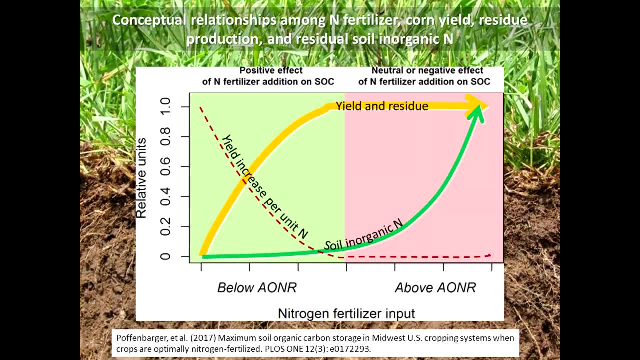 that mythical perfect year that's going to happen next year. right, You want to have enough fertilizer out for that year. So every year you put out enough fertilizer for that one year. that might happen in one in ten years or something if you're lucky. 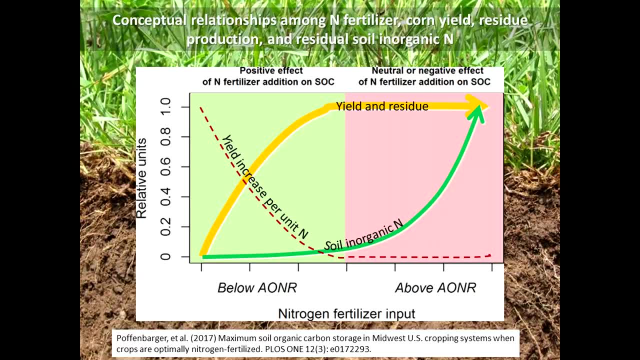 That means the other nine years. you're over-fertilized, So that's a problem we need to deal with, And that over-fertilization is eating up your organic matter as well as your bank account, as well as the patients of your neighbors. 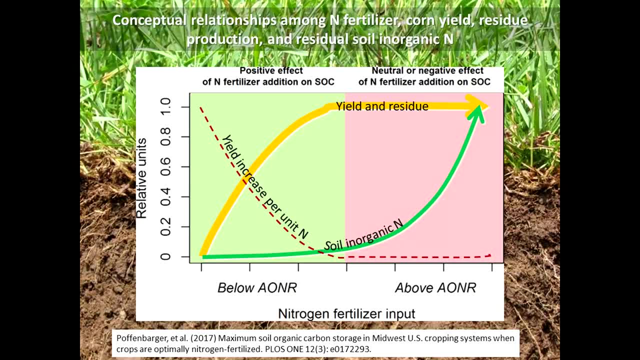 who are drinking the nitrate in their water supply. So the problem with accumulating inorganic nitrogen and eventually leaching it is really a problem of excessive application. as long as that nitrogen is at the right amount, we're not creating much in the way of problems. 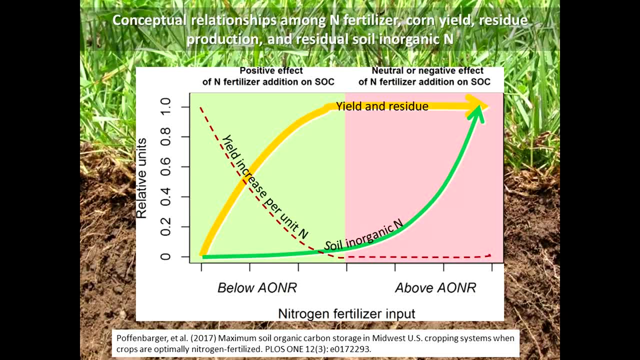 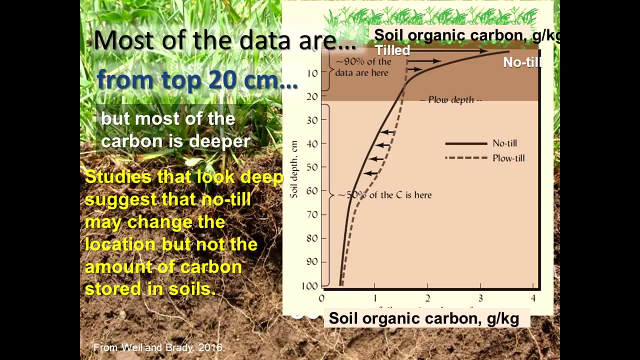 And, of course, the efficiency does go down, which you need to keep in mind. The more fertilizer you use, the less efficient that last bit is, the less you get back for it And you don't want to go all the way to zero and start getting negative. 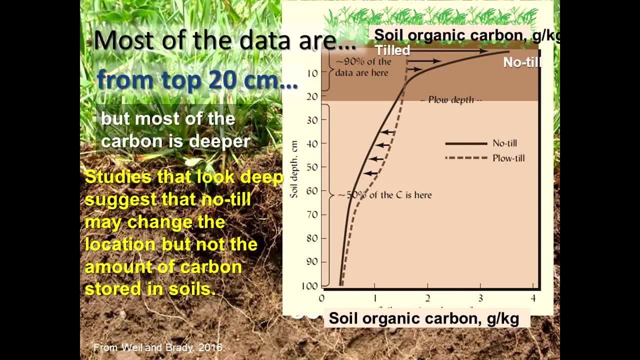 What we found with tillage is when we stopped tilling, we're slowing down that respiration, We're not exposing all that organic matter, and organic matter accumulates. And for a long time we had just solved that carbon problem And the NRCS was all excited. 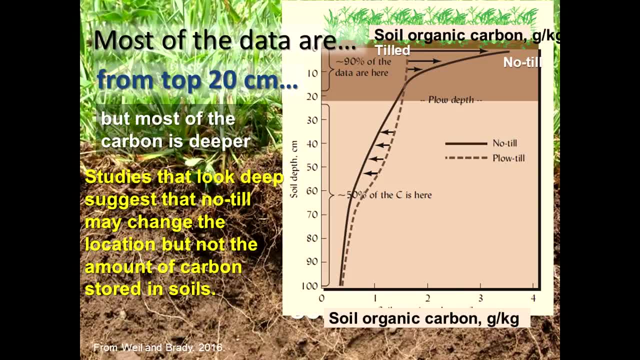 about no tillage and an increased carbon, And almost all our samples were right near the surface And that's where the changes take place first. If you want to see the impact that you're having with your management changes in no till you want to measure it. 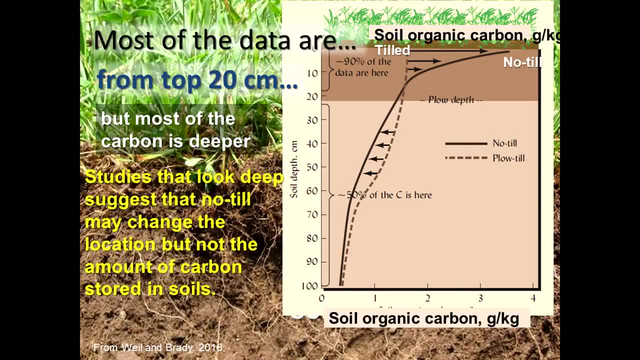 in the top couple of inches. But it turns out that if we take deeper samples maybe we weren't getting that far ahead. We're just not sure on this. Typically we find in no till a lot more carbon near the surface than in tilled. 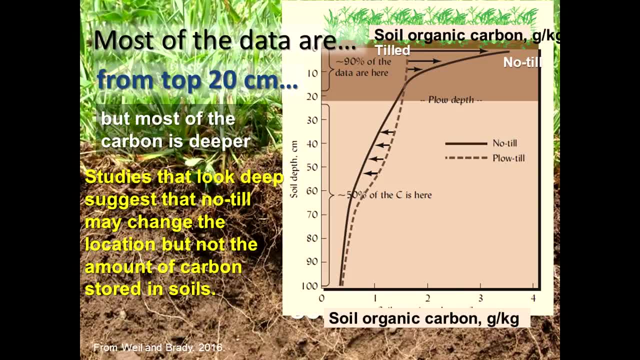 But the deeper we go, sometimes these lines tend to cross. It may be that when the people that are using conventional tillage are forcing the roots to go deeper because that surface dries out And so the deeper roots are putting a little more carbon in there. 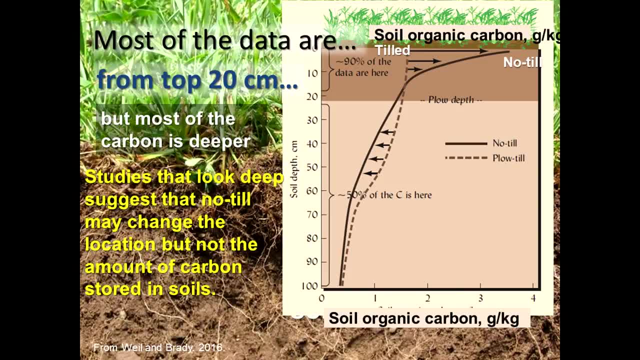 When we go down to like three feet deep- this is in centimeters, so it's a meter. We often find that that difference in tillage in the overall carbon in the whole profile disappears Doesn't mean we shouldn't be using no tillage. 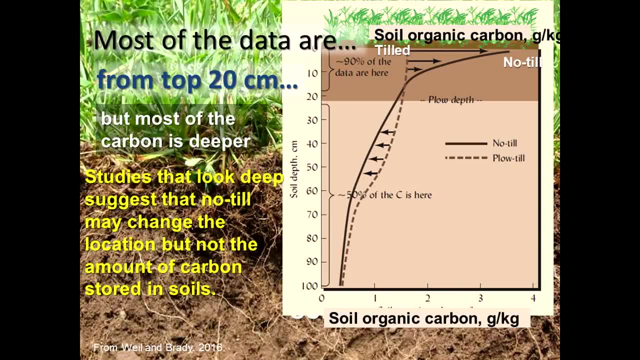 We're improving the health of the soil up here, We're doing a lot of good things. In terms of the total carbon pulled out of the air, it may not be that different Depending on a lot of other factors, So this was a bit of a. 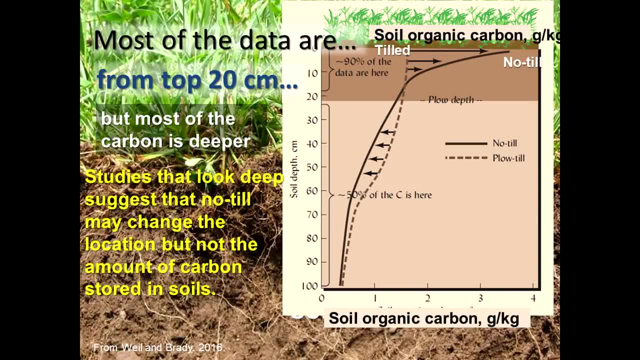 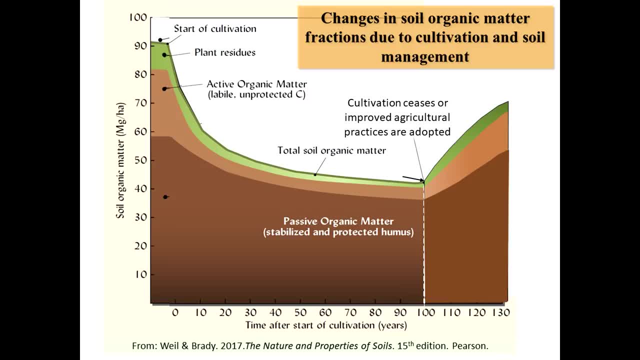 disillusionment for a lot of us in the soil conservation, But this is just a fact. We're out of time, Okay, So I can quit here. I did have a couple of things. I wanted to get to this calculation, See if we have time for this. 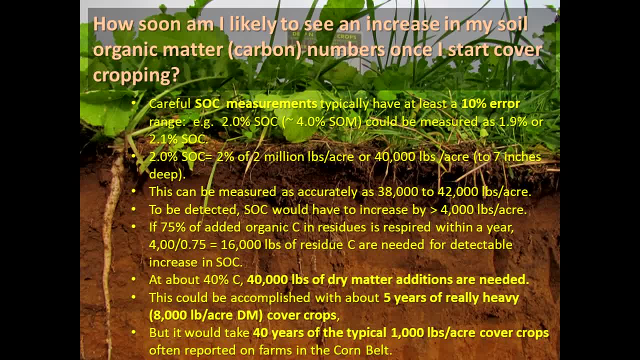 So I think some of us are being a little unreasonable in our expectations as to what cover crops are going to do And, of course, a cover crop. there's huge differences in cover crops- right, The average cover crop. it's a good thing. More and more people 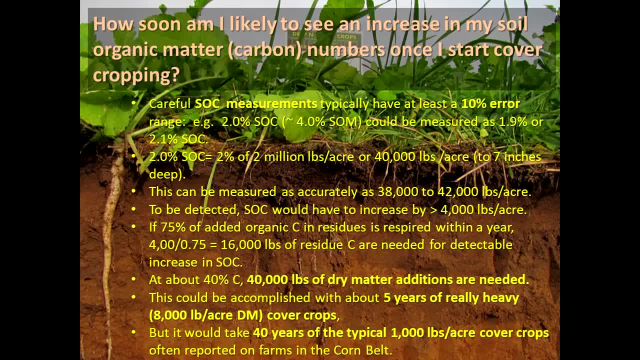 are growing cover crops. I'm guessing that we're up to something like five to ten percent. Does anybody know what the latest statistics are? Anybody have a feel for that in Indiana or Ohio? It's about ten percent in Indiana last year. 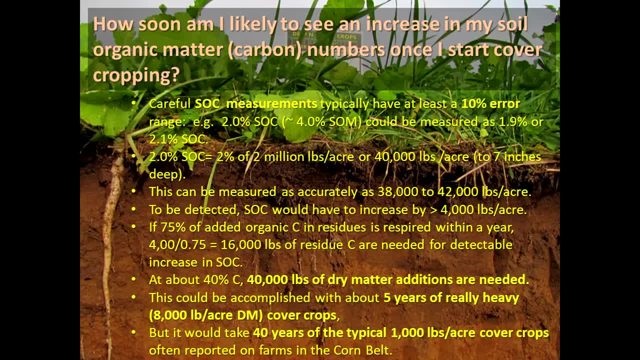 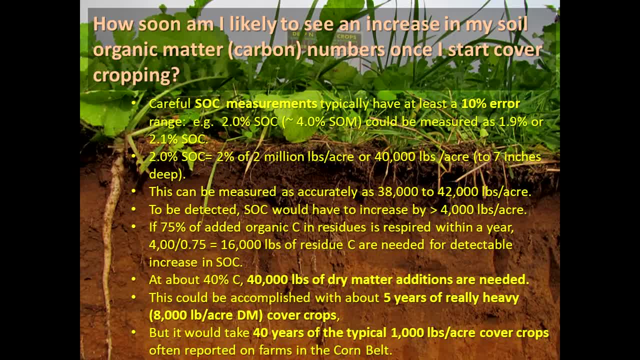 Any other questions? Yeah, So so many people have questions about acreage. Yes, Just about a million acres, About a million acres of cover crops in Indiana. So that's my feeling is that it's pushing up around the in different states. 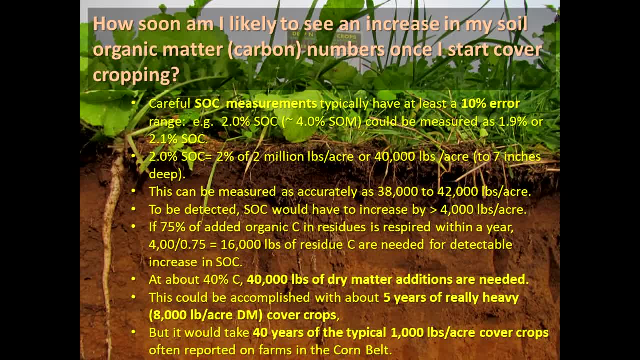 Indiana's probably ahead of the game. It's a pretty good state in that regard. But how good are those cover crops? You know what's the biomass? How much can you really build organic matter with them? So, given what? so much of it, and it's so variable that you're lucky if you can measure it. 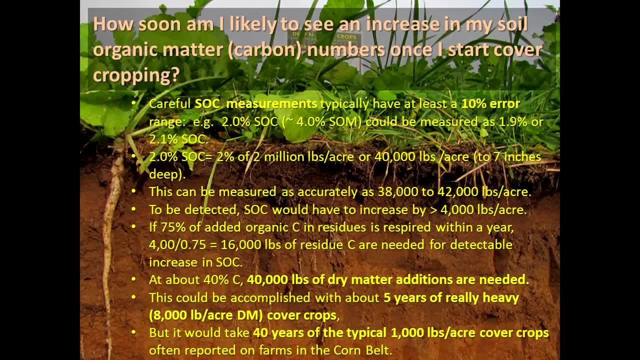 within 10% of reality, so there's going to be some error. so let's take a soil that's 2% solar organic carbon, which would be 4% organic matter roughly, which translates to about 40,000 pounds of carbon. given that error, you can only: 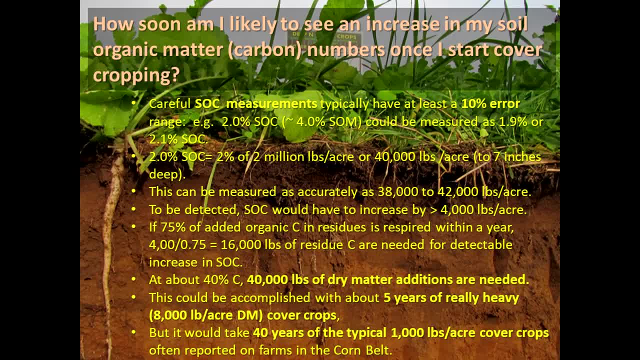 measure between someplace between 38- 42 thousand. so in order to measure a difference, in order to see that you've increased your organic matter from cover crops, you're going to have to increase it for that soil to fairly typical soil around here by about 4,000 pounds of carbon per acre. now remember about 75%. 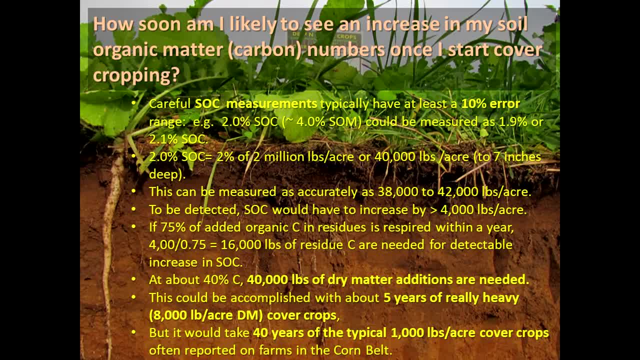 and this depends on who's doing the respiring, but about 75% of the carbon you add is being inspired. so to get to 4,000 pounds, that's a measurable increase- you're going to need to be adding about 16,000 pounds of carbon. 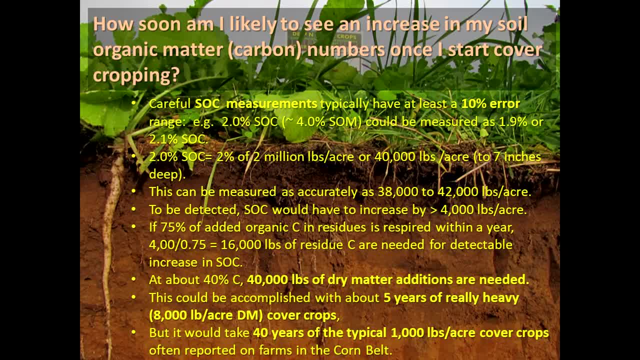 in residues. now remember that residues are only about 40% carbon, so that's about 40,000 pounds of dry matter in order to just begin to see a change in soil organic matter. so you can do that in about four or five years of a really 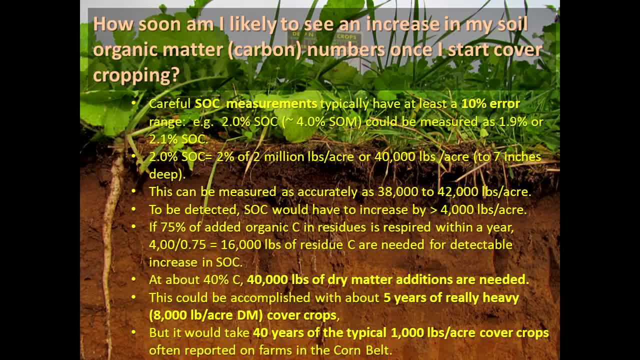 big cover crop. I mean, that's the cover crops that you let the ride go and you've got a huge. I don't know how many of you measure your biomass, but 8,000 pounds, 10,000 pounds, those are really heavy cover crops and most farmers aren't brave. 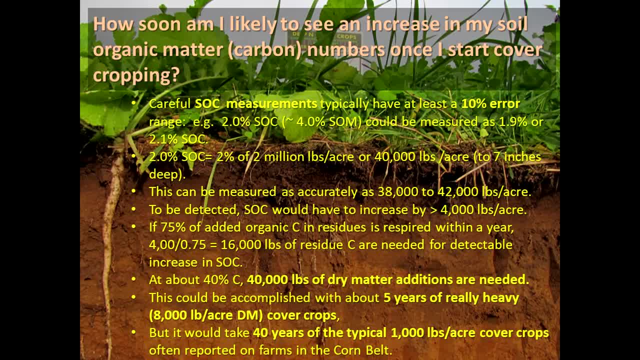 enough to try to deal with that much. we now know- I'm sure this has been covered- that the easiest way to deal with it is to plant right into it while it's still alive, and that works really well with most equipment. so for most of our typical cover crops that I see out there that grow about six, eight inches tall, 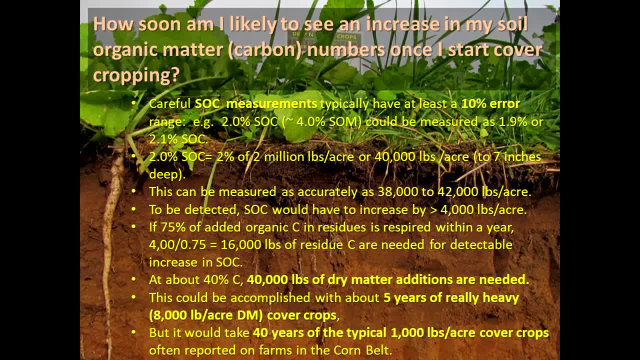 and then they get killed. early in spring they're probably producing less than a thousand pounds of dry matter. so at that rate it might take, you know, 40 years before you had a measurable increase in total soil organic matter. you can see the direction you're going in by measuring the active component. but